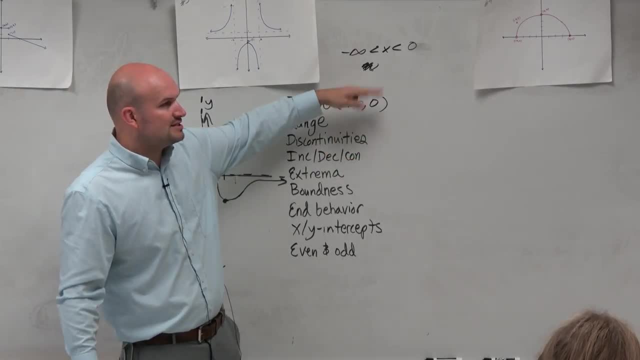 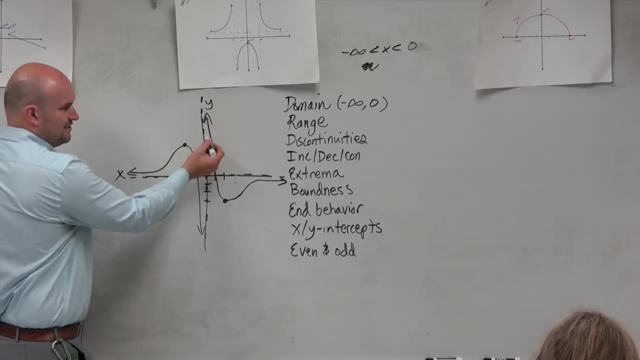 I will say, though, this is the preferred method of using interval notation. It's basically just taking the left, Left to the right. Now we have this other part of the graph where you can see well, this graph looks like it kind of starts at 0.. 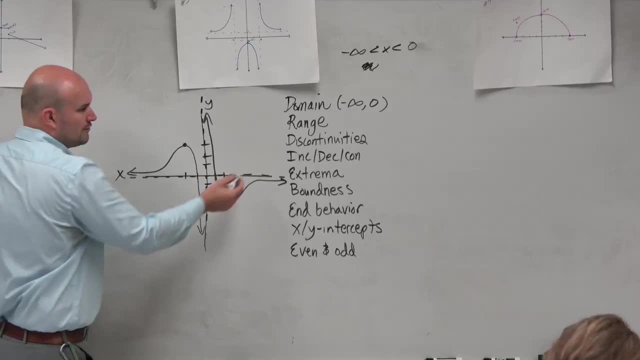 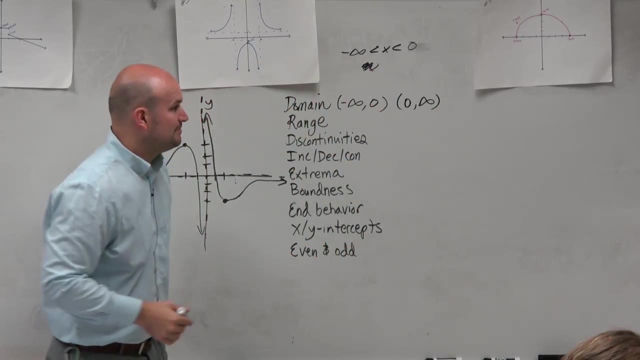 0 is not defined, but it goes from 0 all the way over to, and it's going to continue going to the right to infinity. Now, some people just like putting a comma between those two. Mathematically we know that these two domains 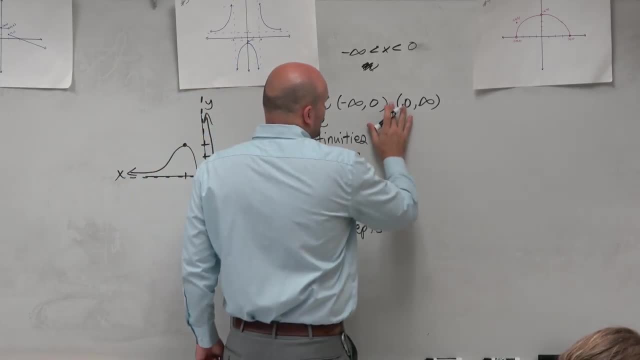 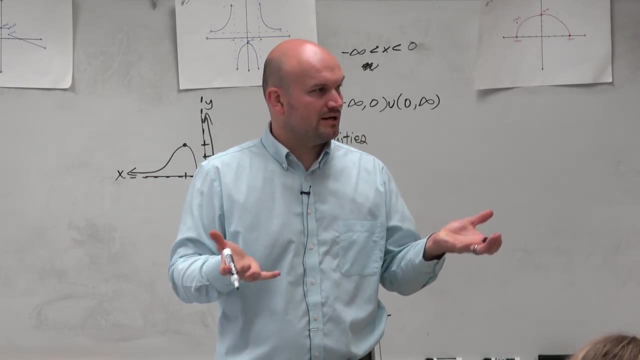 are kind of like together. So if you guys remember, in sets we're going to say, well, what's that union symbol? A lot of times, remember, we use the union symbol like the or, which is like a combination of the two. 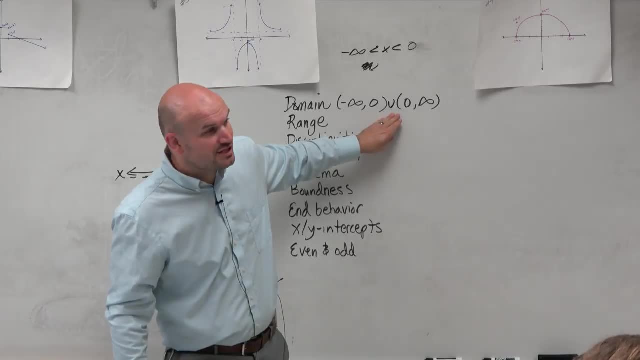 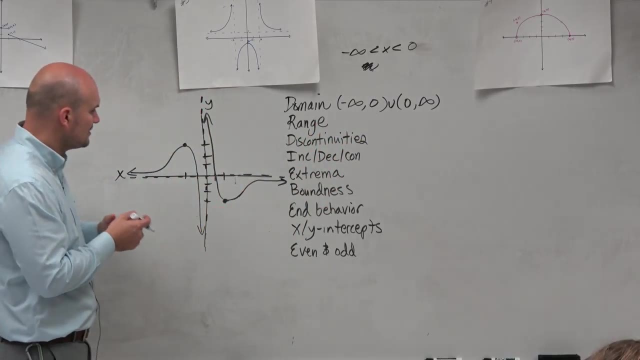 intervals. So you guys will see that a lot You don't need to use the union symbol. but I don't want you to be like: what's that union symbol? It just means you're connecting those two domains. The range is kind of interesting. 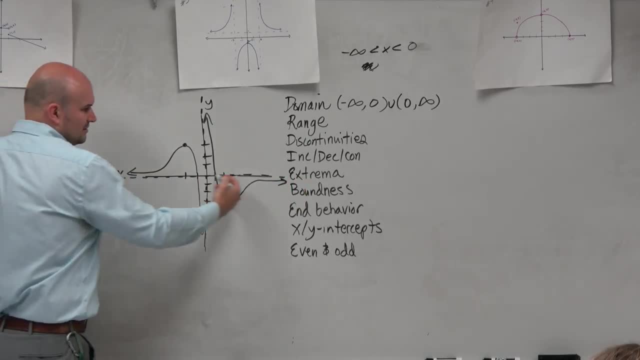 You guys can see that there is a horizontal line that the graphs are approaching from the left to the right, But also the graphs cross that line Right. So it's not undefined for that given value. You guys see that It's not undefined at that line. 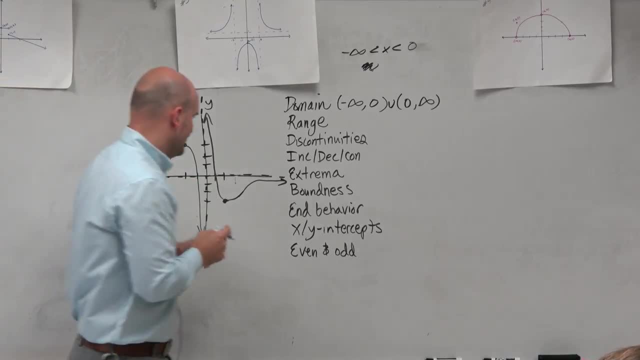 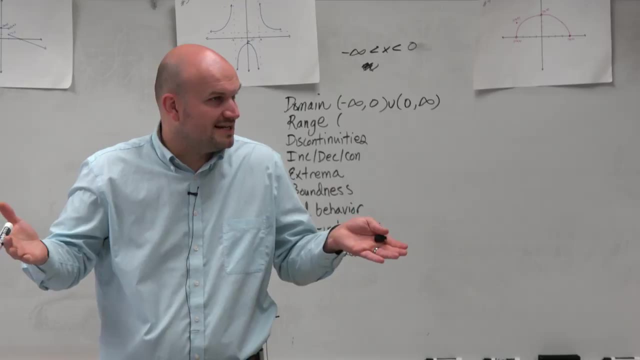 It's approaching it, but it's not undefined, And we'll talk a little bit more about that in a second. So the domain is basically how far left to how far right the graph goes minus any discontinuities. The range is basically saying how low is the graph going. 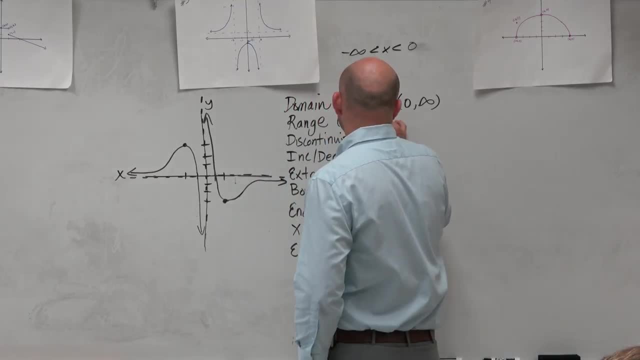 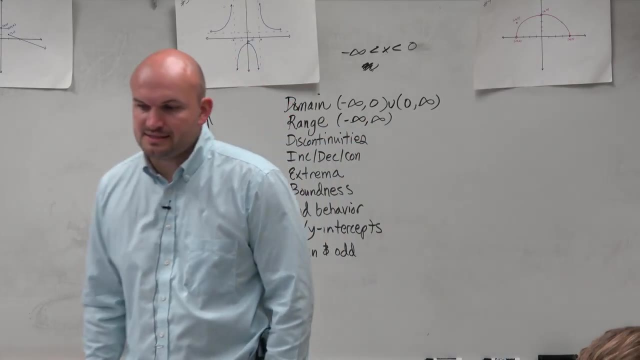 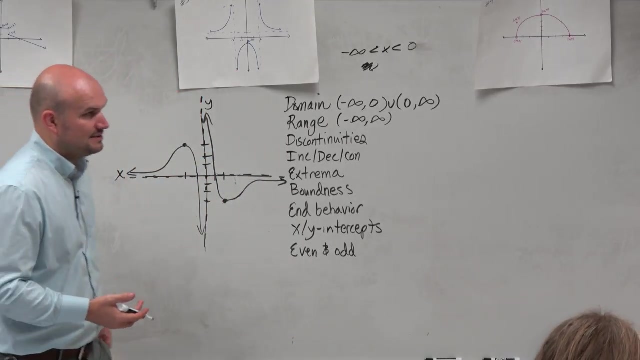 to how high is it going? And in this case we can say it's negative. infinity to infinity. All right, Now discontinuities. Discontinuities is basically saying we're asking: one, is the graph continuous? And then, two, what type of discontinuity is it? 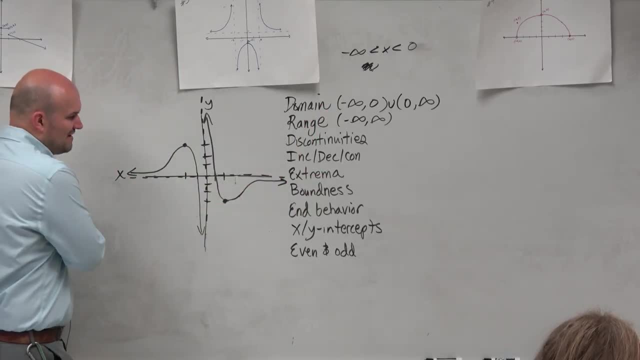 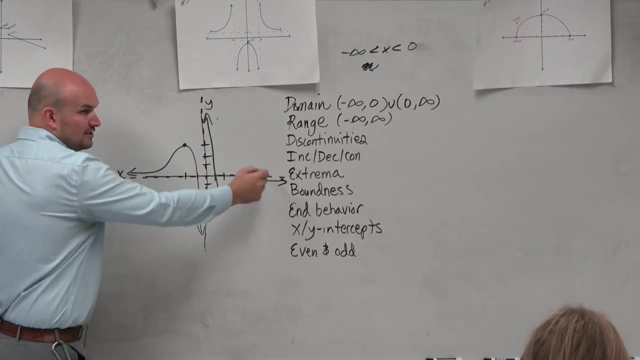 All right. So the way to test again: if a graph is continuous, can you draw the graph without lifting up your pencil? And I can't, because I have to somehow cross this asymptote, So I have to go over there. 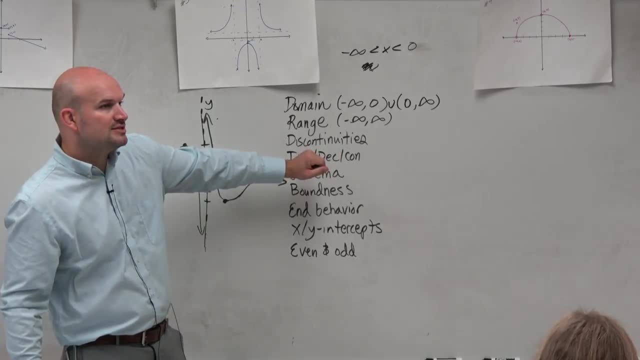 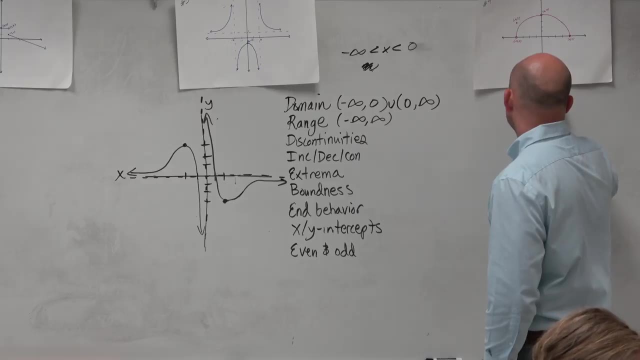 So it's definitely discontinuous. But now we want to be able to identify the discontinuity, And I guess I didn't, So I got room here. So there's a couple different ways, There's a couple different types of discontinuities. 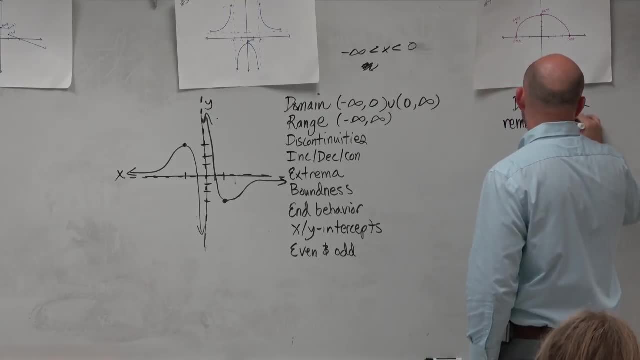 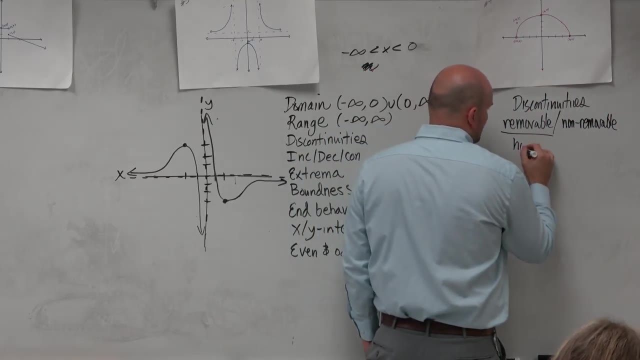 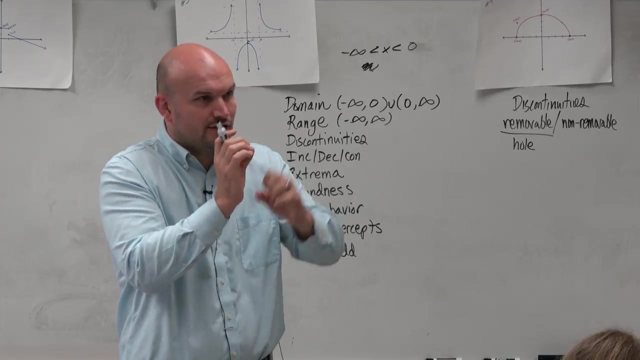 There are removable and non-removable. OK, If it's a removable, it's a whole, all right. And that basically means it's like a vacant portion of the graph, right? You're looking at the graph and it's just like a vacant dot. 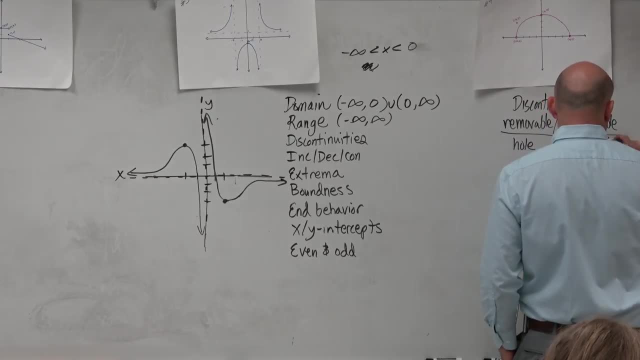 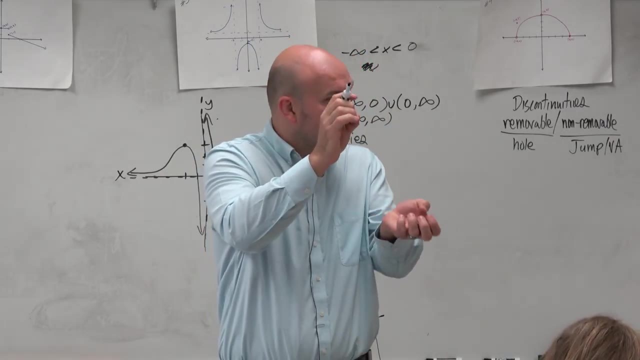 Non-removable would be a jump or a vertical asymptote. So a jump is basically going from one part of the function, jumping to another part of the function, or two different functions, like a piecewise function. You're jumping from one function to the next. 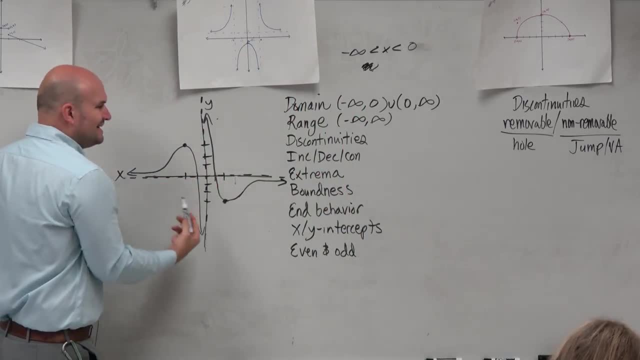 Whereas a horizontal asymptote. a lot of people say, oh well, you're jumping, Yes, but remember, the horizontal asymptote is an undefined value where the graph is approaching. all right, And notice, I'm talking about vertical asymptotes. 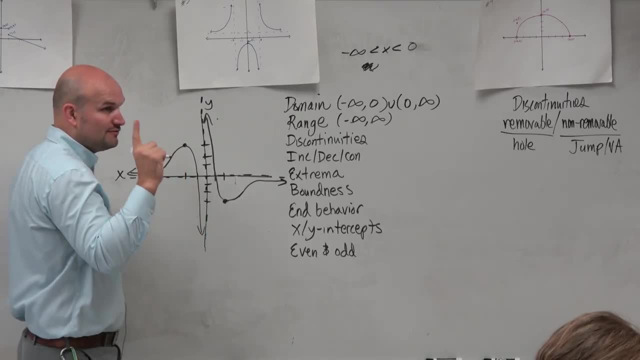 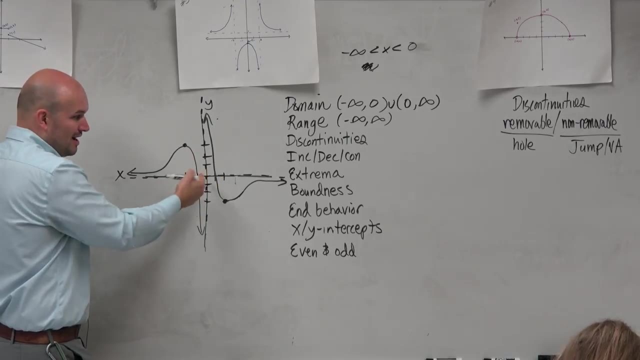 I didn't say horizontal asymptotes, because one, we're looking for discontinuities of the domain and second, vertical Horizontal asymptotes. Horizontal asymptotes can cross. This is an example of a graph that crosses the horizontal asymptote. OK, 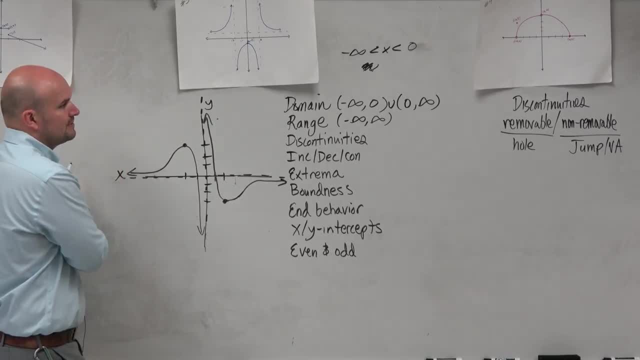 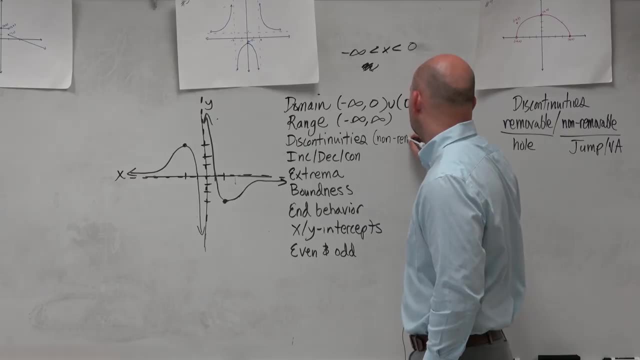 Horizontal asymptotes are not discontinuities, but vertical asymptotes are. So this is, since it's a vertical asymptote, we could say that it's a non-removable vertical asymptote, And the best thing to do when you're a lot of times when 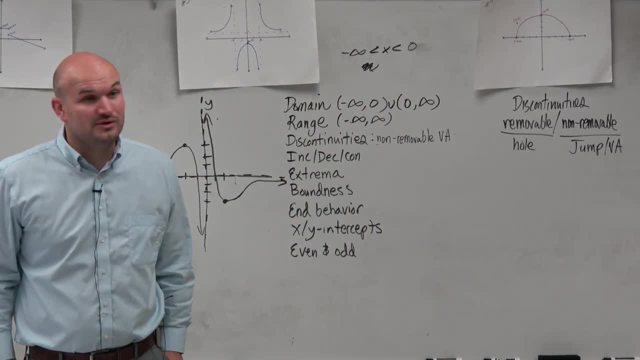 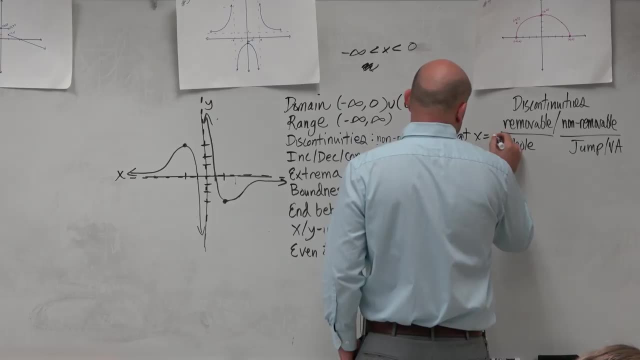 I'm asking about discontinuities. I might say: where does that discontinuity exist? Where is that discontinuity? And therefore you'd have to say: well, it exists at x equals 0. Because when at x equals 0, that's. 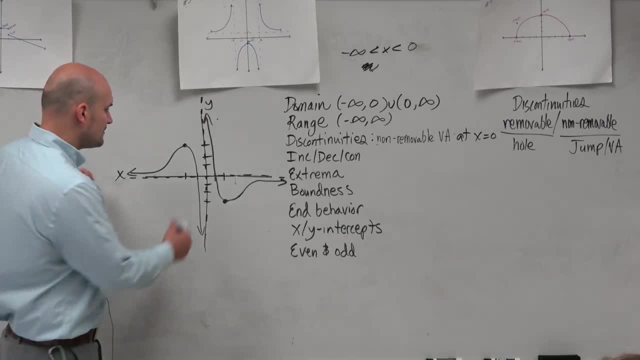 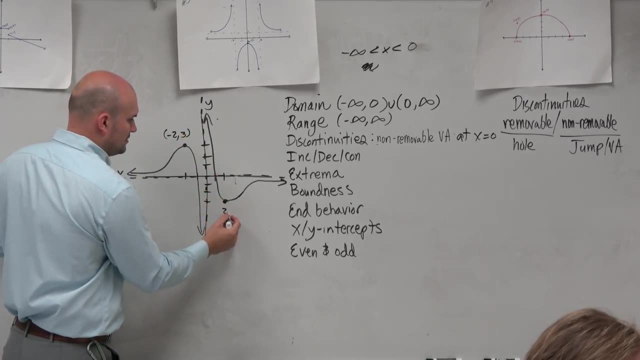 where the graph is broken up. OK, Now, I didn't list these points, so let's go and do that. 2, 3, 2, negative, 3.. OK, increasing, decreasing constant. This one gets a lot of students. 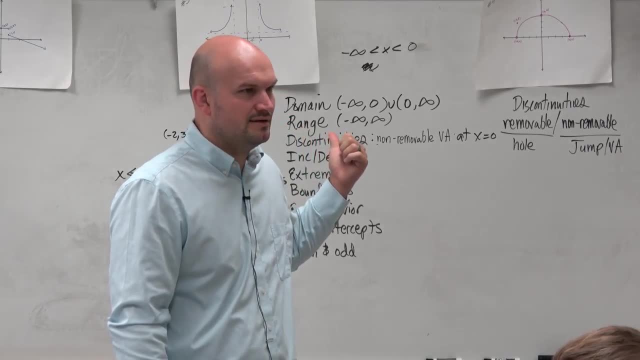 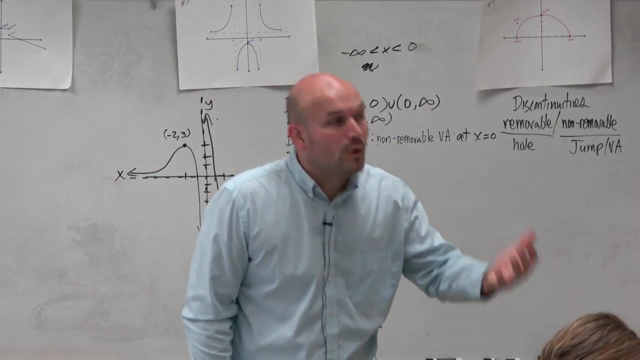 And I don't think any group did any increasing decreasing up here, did they? Not one group? I need to get you guys All right. so increasing decreasing constant is basically asking us: when is the graph Again? I'll say it one more time. 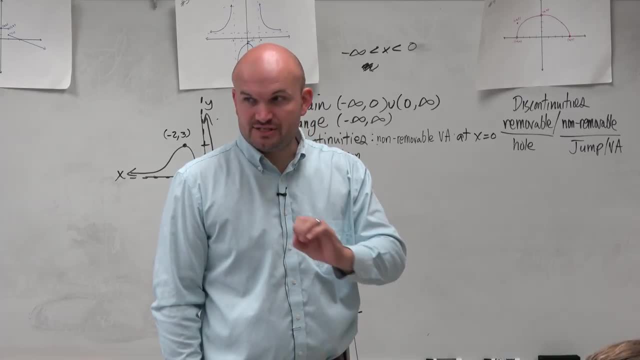 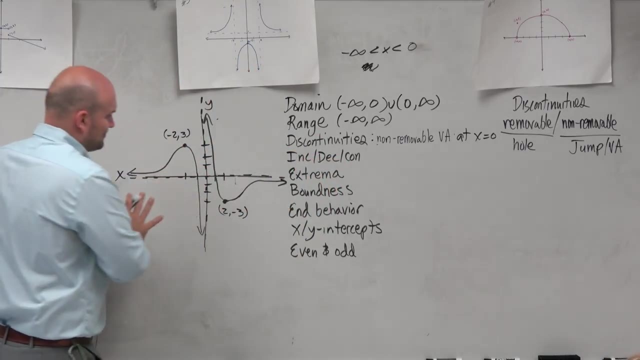 When is the graph? increasing, decreasing or constant? So now what we need to do is we need to put our hats back, like our thinking hats as far as looking at a graph. As we read a graph from left to right, the x values is basically: 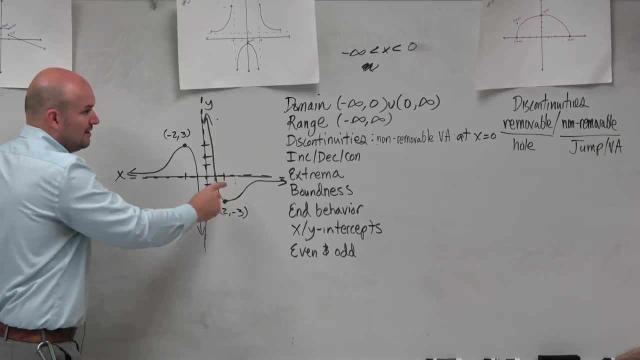 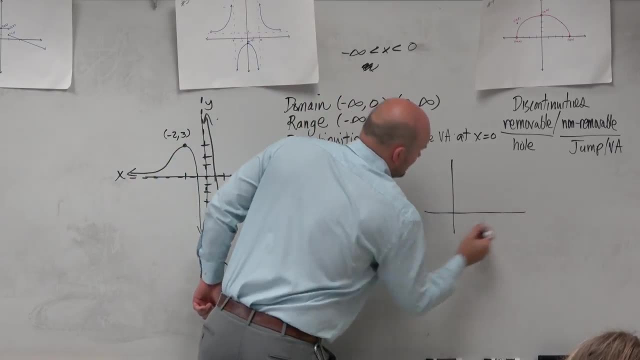 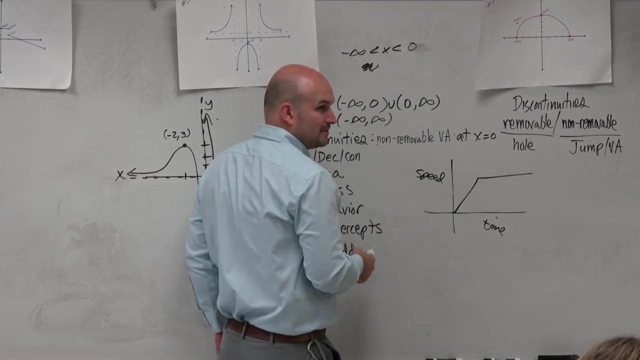 like x is basically telling us the when And the y is basically telling us the what. right Here is like you're traveling. The easy example I think of was like let's say here's time and let's say here's speed. 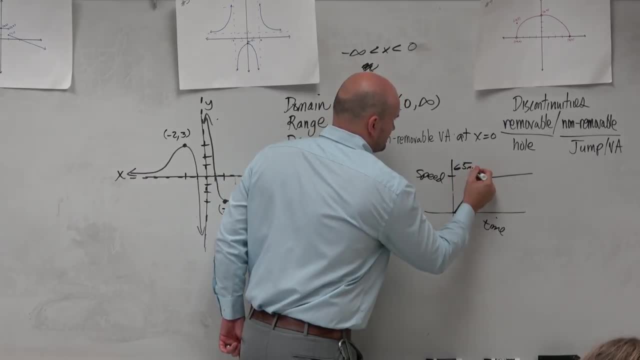 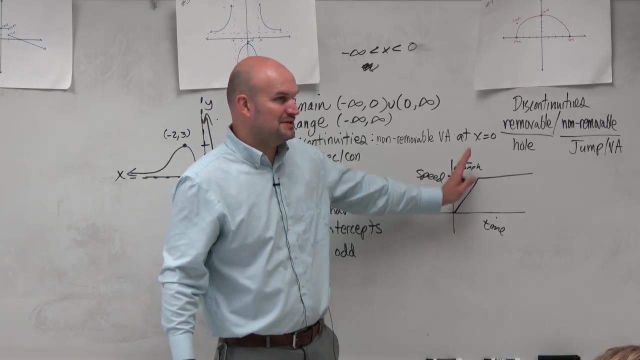 And let's say here's 65 miles per hour. You start at 0,, you get in your car, you drive to the highway at a constant acceleration to get to 65 miles per hour, And then now you're on the highway. 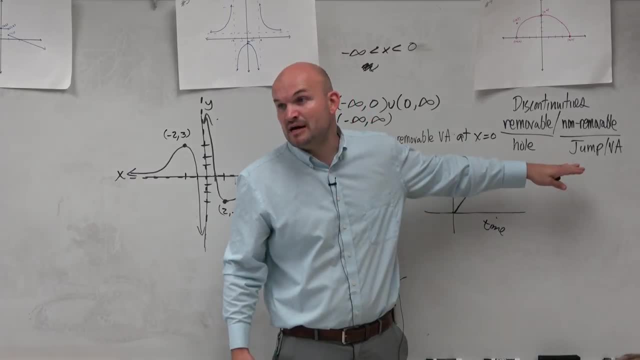 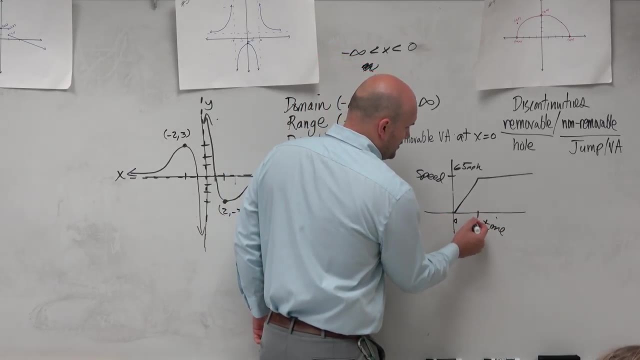 and you put on cruise control and you stay at 65 miles per hour. And if I say, when were you increasing your speed, you would say: well, you increased your speed from 0 to 5 minutes, Don't you guys agree? 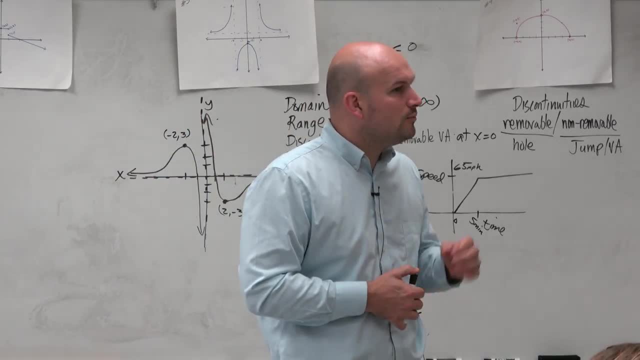 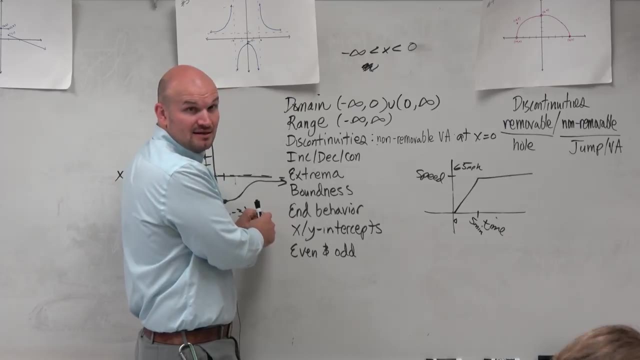 You wouldn't say: oh, I increased my speed from 0 to 65.. No, when did you increase your speed from 0 to 5?? The when is the x values. Does that make sense? Not the y values? The y values is telling you what the speed. 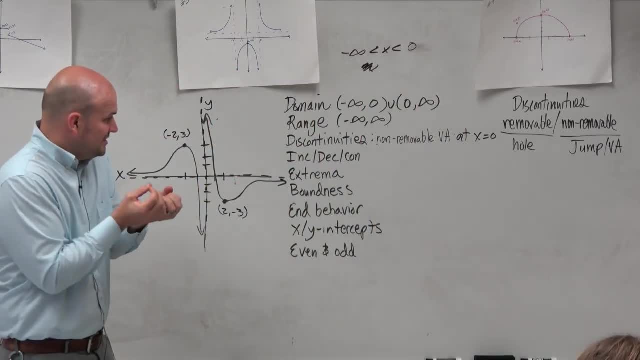 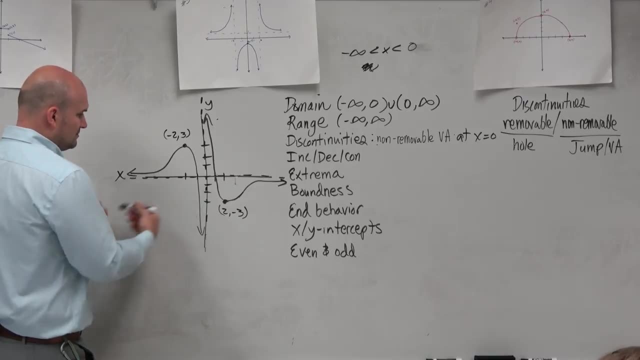 And that's different because I can phrase my question differently. So if I'm asking you for the increase, I'm basically saying: when is the graph increasing, When? So we look at this and we say, well, starting from the farthest left, as we 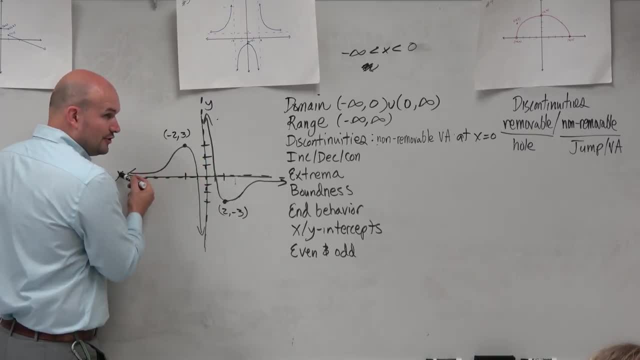 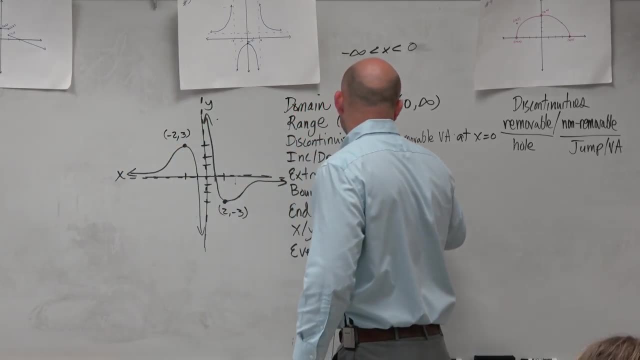 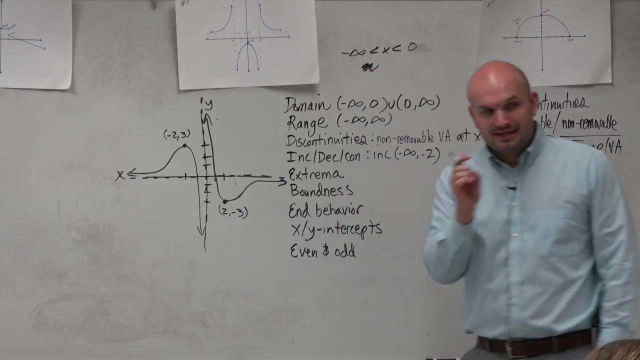 go from negative infinity all the way to negative 2, the graph is increasing. Am I asking how much is the graph increasing? No, So we can say the graph is increasing on the interval: negative infinity to negative 2.. OK, Increasing, decreasing intervals are intervals. 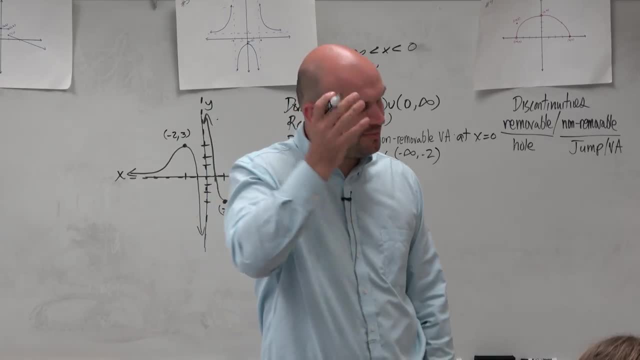 They're not coordinate points. A lot of students will mix them up and they'll like: oh, it's a coordinate point. No, Don't say it's increasing from negative infinity to negative 2, 3.. That's a coordinate point. 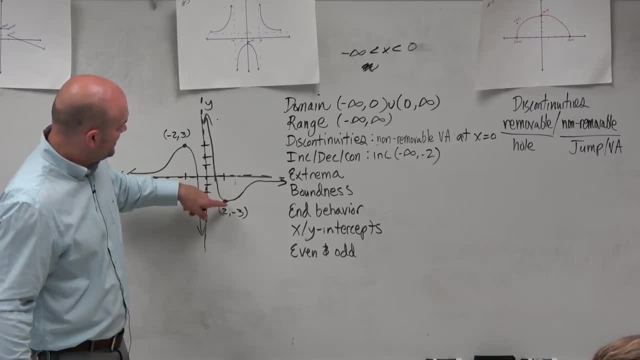 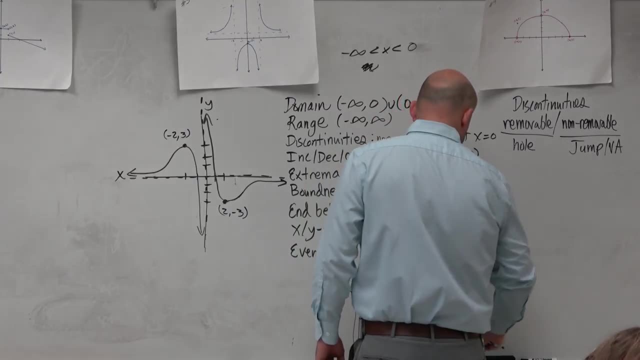 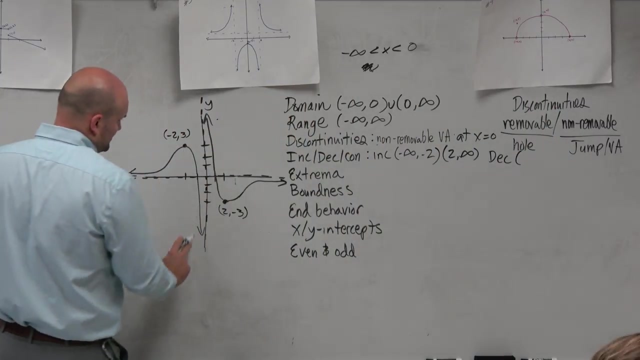 So these are intervals of increasing. You guys can also see from the interval 2 to infinity that the graph is increasing, And then we can say the graph is decreasing on the interval Negative 2 to 0, and on the interval 0 to 2.. 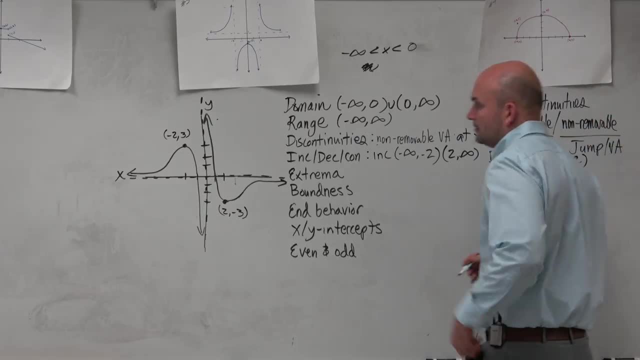 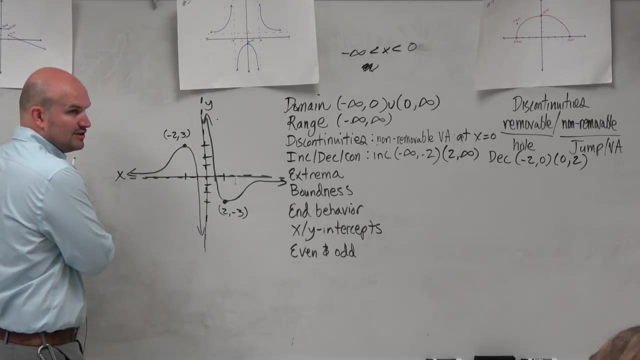 Now let me reiterate a couple points here. What's wrong with me saying, from negative 2 to 2, that the graph is decreasing, Because it's decreasing here and it's decreasing there. So what's wrong with me saying just it's decreasing. 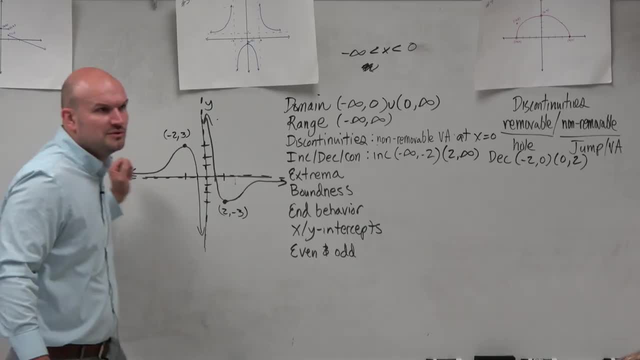 from negative 2 to 2?? Because what, Yeah, they're not connected. So if you say it's decreasing from negative 2 to 2, it's decreasing from negative 2 to 2.. It's decreasing on the interval negative 2 to 2.. 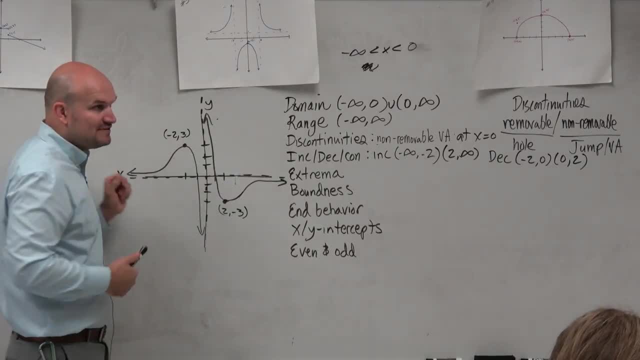 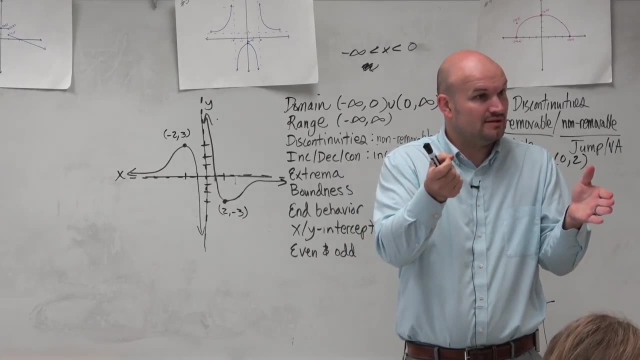 Wouldn't you then assume then at 0 the graph is decreasing? If you say on the interval negative 2 to 2 the graph is decreasing, that tells me that 0 the graph is decreasing, But 0 is undefined. So that's why we have to separate that out. 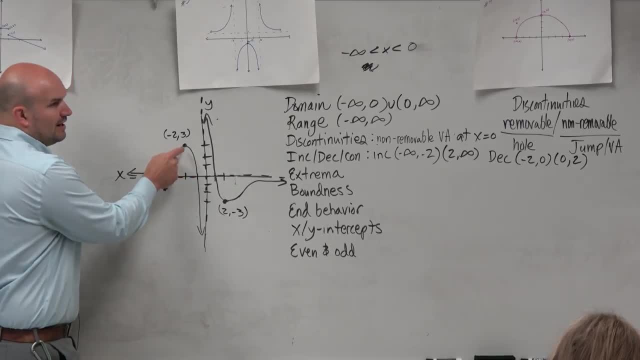 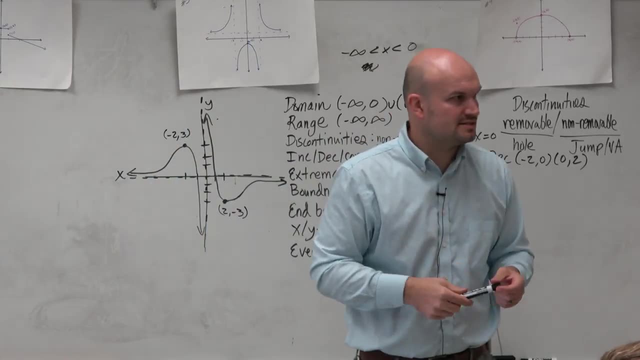 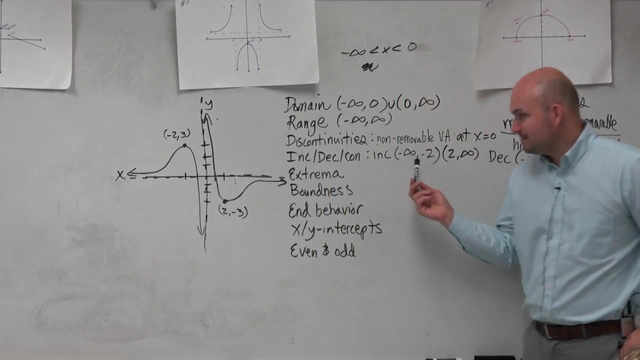 The other thing is: why don't I use an included symbol here? If negative 2 is a point, why don't I use the bracket instead of the parentheses? Anybody have an idea? That's OK. So the reason why, when we're talking about it, 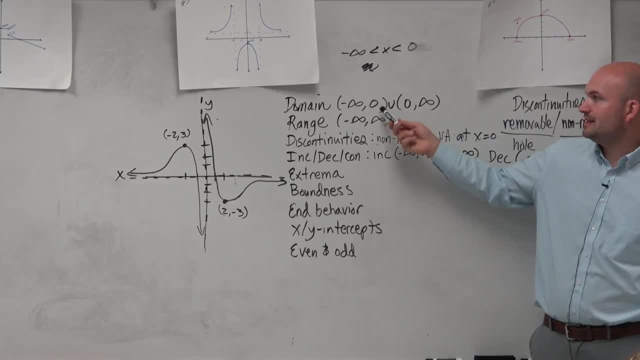 because in domain and range, if a point is included, see the asymptote- is not included. because 0 is not a point, so that's why it's a parentheses. Infinity is not a number, so that's why it's a parentheses. 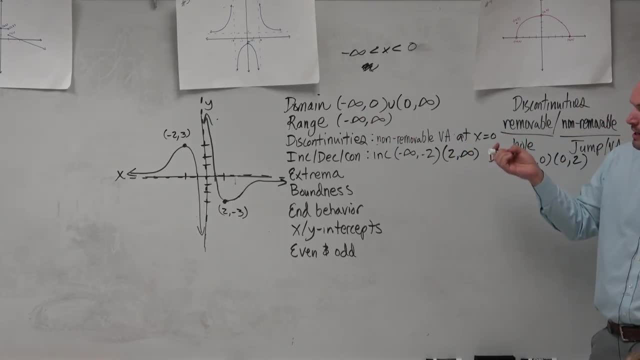 But when a point is included, then we do want to include them, And I guess I forgot to mention that on there. So just remember, guys, if a point is on the graph, you want to use brackets for domain range, But for increasing, decreasing we. 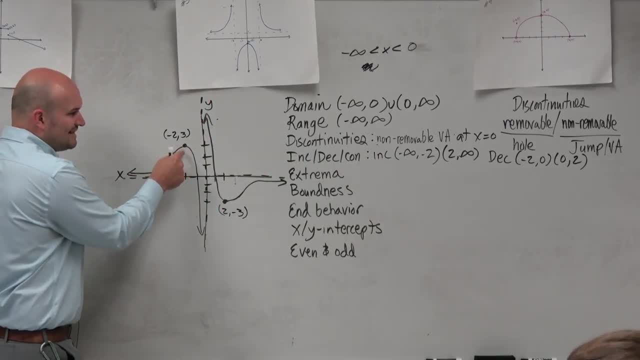 don't want to really use that because look at the point: negative 2.. At the x value, negative 2, if you use a bracket, that means negative 2 is increasing or is negative 2 decreasing. Which one is it? 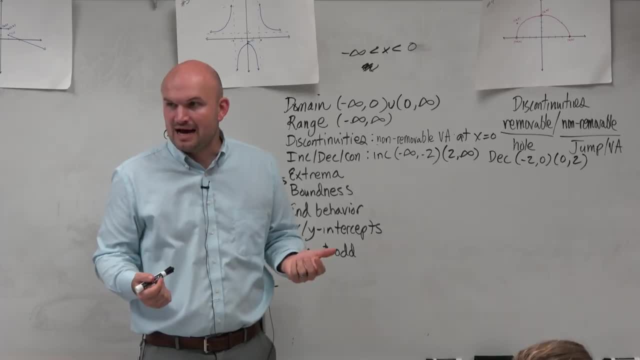 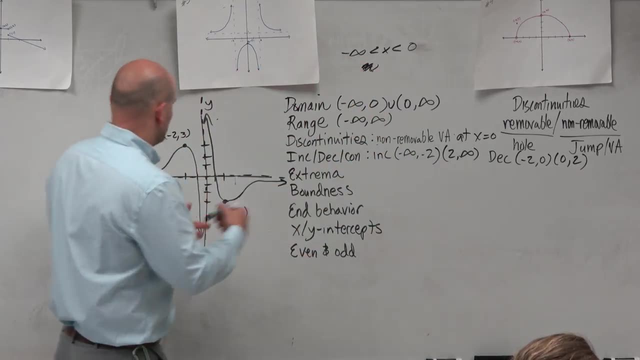 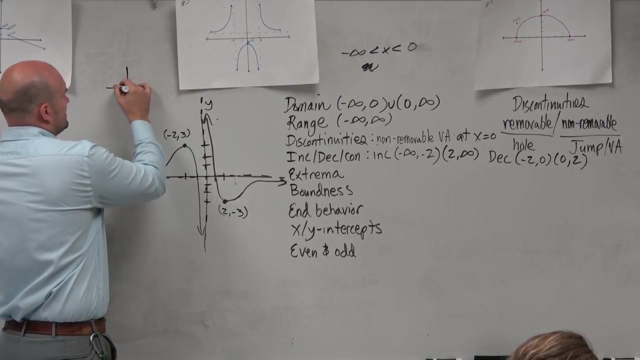 You can't be both, You can't be increasing and decreasing at the same time. So that's why, when we're talking about increasing, decreasing intervals, we're always just using parentheses And just real quick, guys. Let me, for instance, if I looked at, if I was going to say: 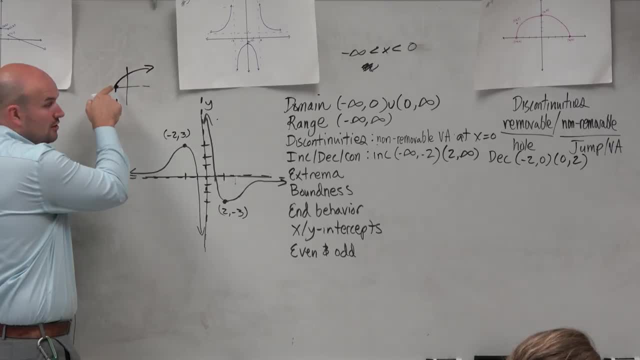 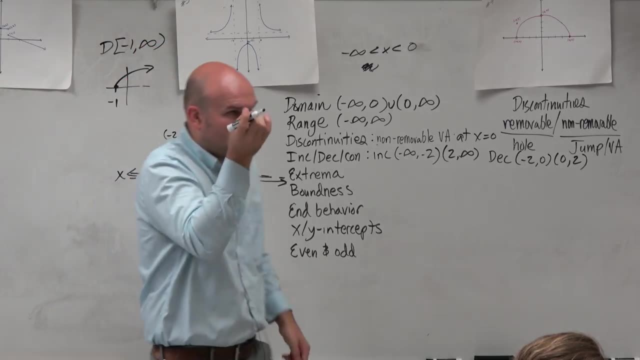 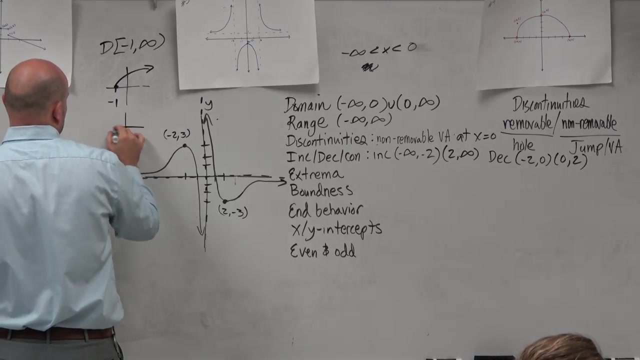 what is the domain of this? See how 0 is included or negative 1 is included. So the domain of this one would be negative 1 to infinity. Do you guys see why I'm using that? However, if it's like a open circle, attention, teacher. 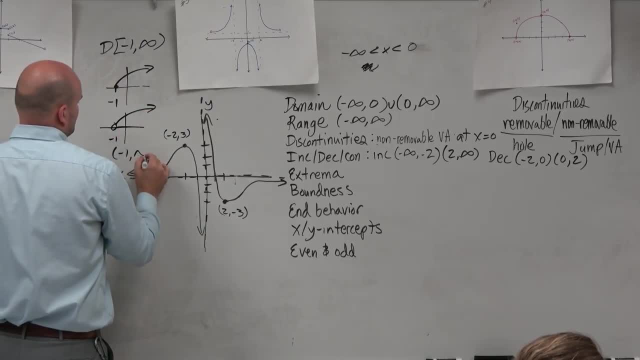 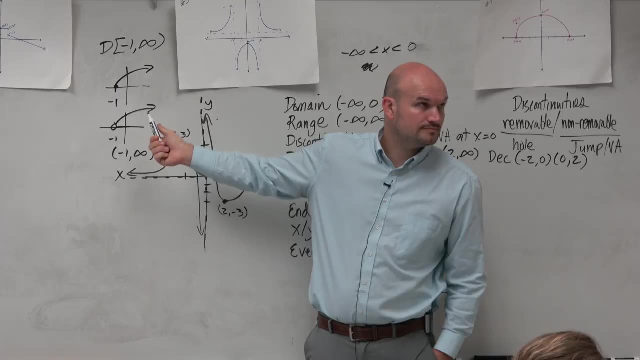 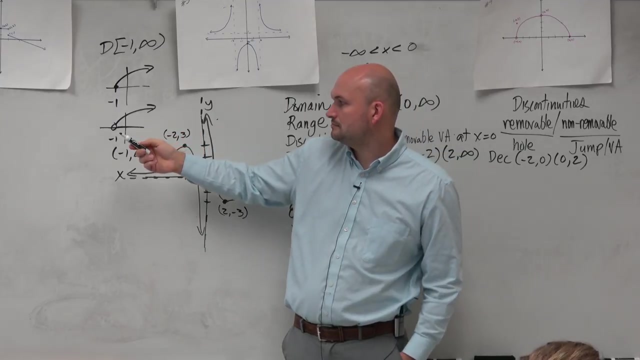 to students At this time. please release all juniors to the auditorium. Hold on a second juniors. I'll finish All of their belongings at this time. Teachers, please release all of your juniors to the auditorium with all of their belongings at this time. 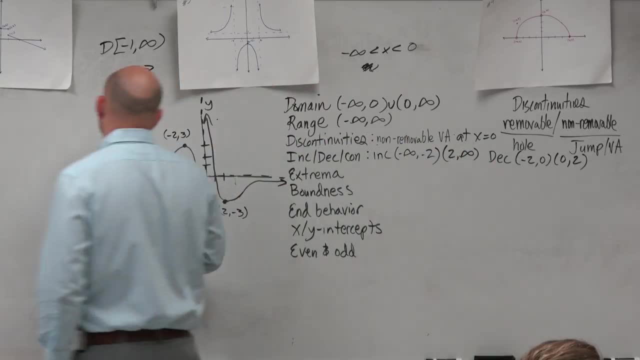 Teachers that only have junior classes: please accompany your juniors to the auditorium at this time. Teachers, if you have other classes in your room, please stay with those students at this time, OK, So just notice the difference, guys. If it's included, you're going to use brackets. 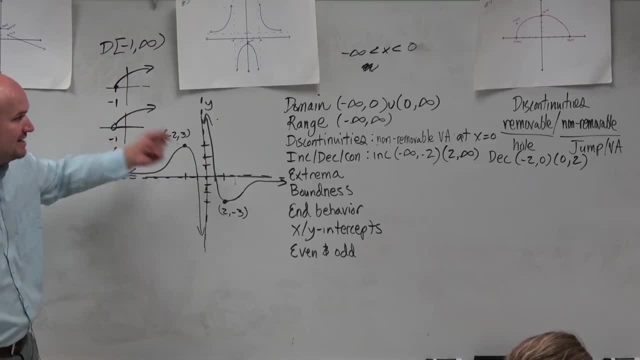 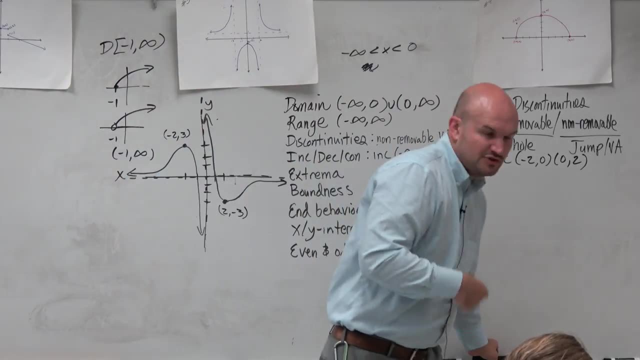 If it's not included, like as a whole, or if it's an asymptote in our case. that's why we're using the parentheses, And this is for domain and range. I forgot to talk about that, so that's why I'm going back to it. OK, 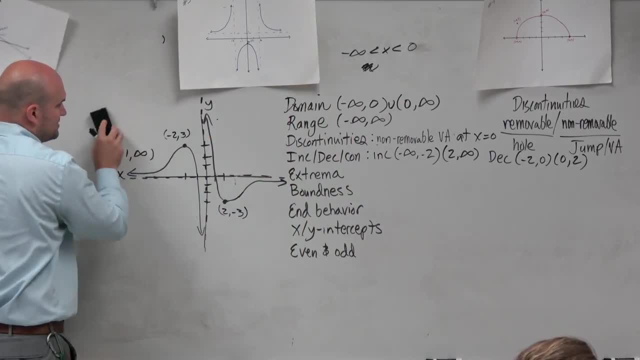 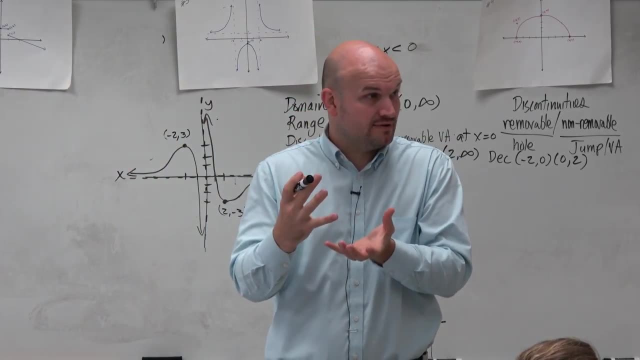 Juniors, if you'll just wait, I'll finish this up real quick, Because I have something I want to tell you as well. All right, Let's talk about extrema. Extrema is basically saying like the highs and the lows of the graph, OK. 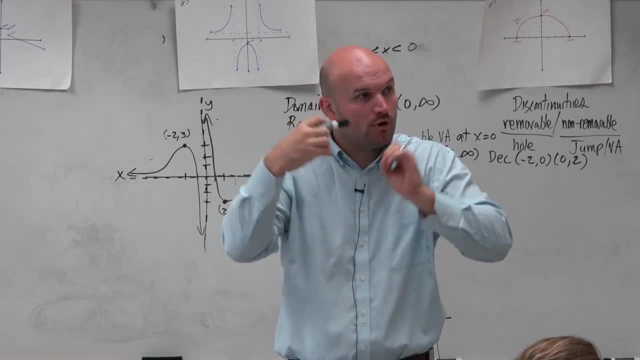 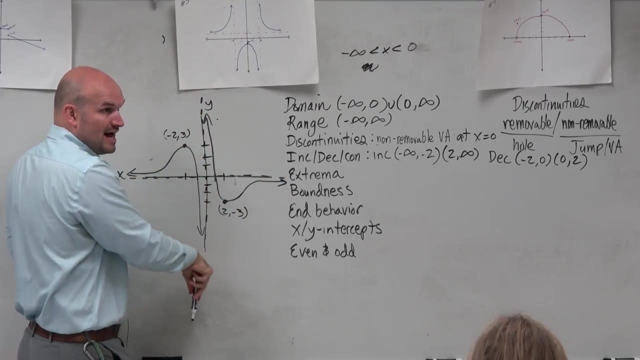 So, basically, is there a point that is a high, like a maximum or a minimum, And if you guys look at this, you can see that this graph continues going up and it continues going down. So there's never going to be a point, that's always. 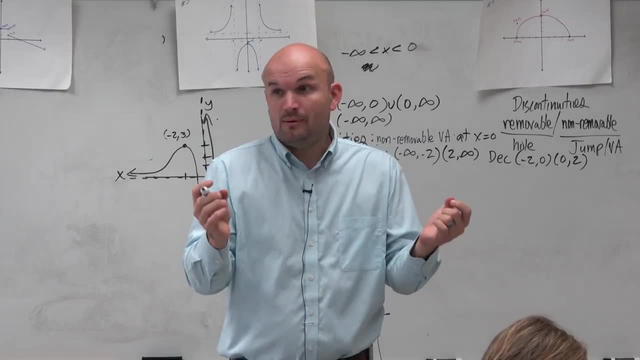 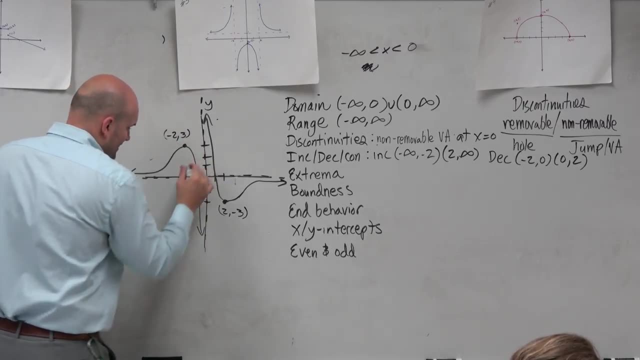 going to be the highest right. Would you guys agree, However, if you were to take like a camera and like zoom in on this graph and let's say you just zoomed in right here? So, on your zoomed in lens, all you see is this: 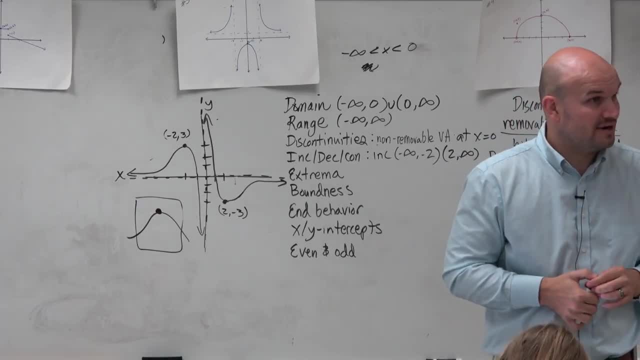 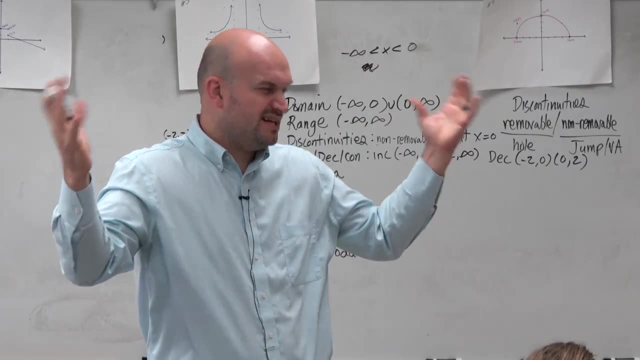 Is there now a maximum point? Yes, Yes, right, But that's relative, to like what you're looking at, right, Because if you zoom all the way out and look at the grand scheme of the graph, then it's not a maximum. 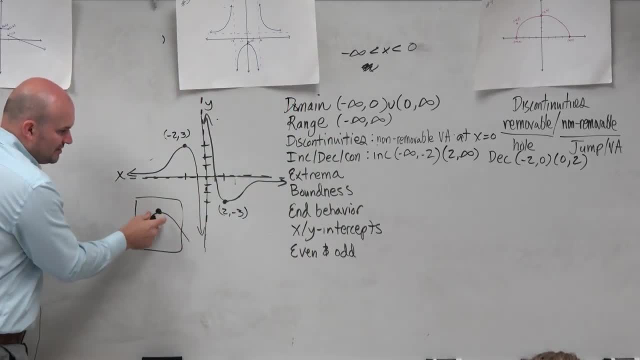 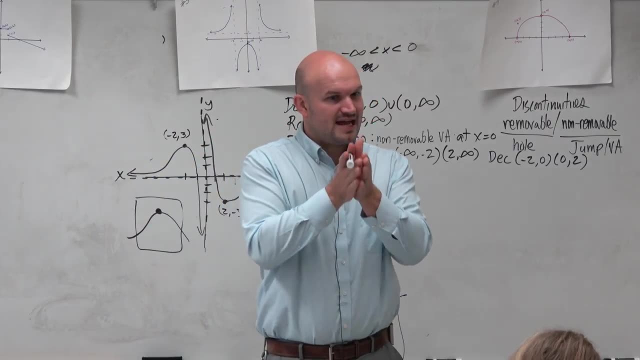 But when you zoom in relative to what you're looking at, you guys can see that it's a maximum And a definition of a maximum. the reason why you guys are saying, yeah, it's a maximum, the definition of a maximum point is every point to the left and every point to the right. 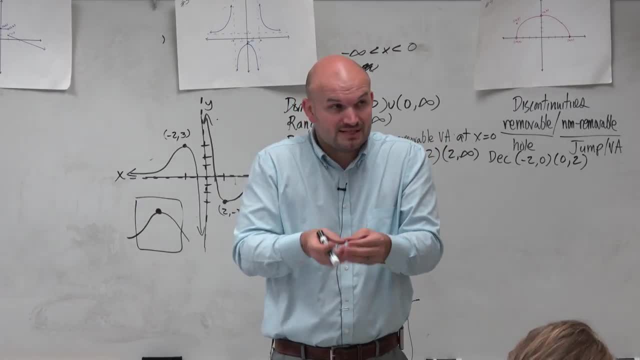 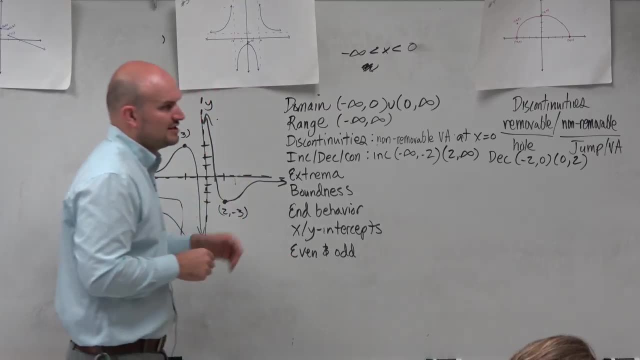 is going to be below The definition of a minimum point is every point to the left and every point to the right is going to be above Right Juniors. actually, by the way, I'll just let you guys go because this is going to take a little bit longer. 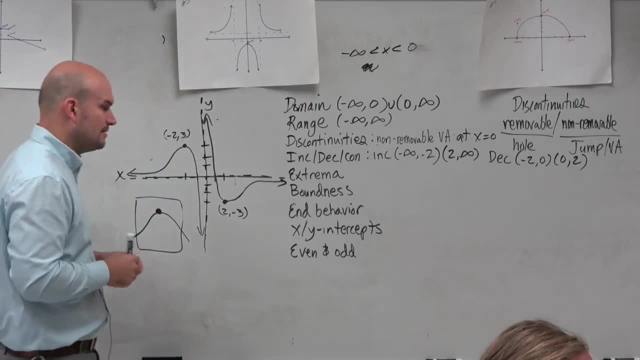 Just make sure you guys have the homework and then obviously, get the notes which you need. OK, All right. so therefore, this is the maximum, But it's not the highest absolute maximum. It's what we call a relative maximum. 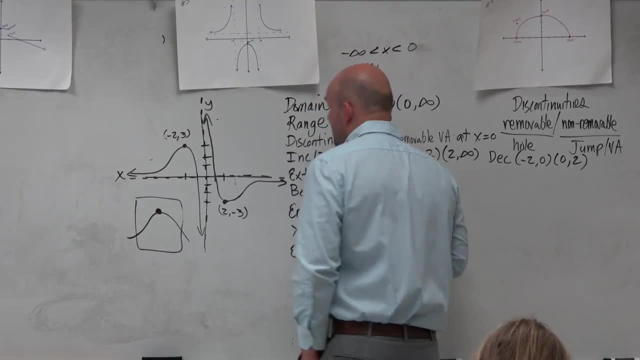 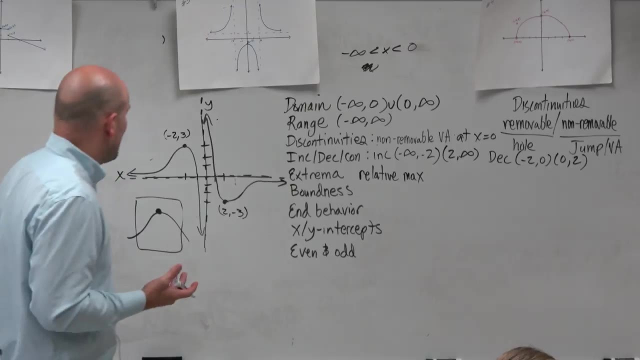 So we'd say a relative max. Now could we talk about location as well as values. Could we say that there is a relative max at x equals negative 2? Like, would that tell you where the maximum value is? Yes, 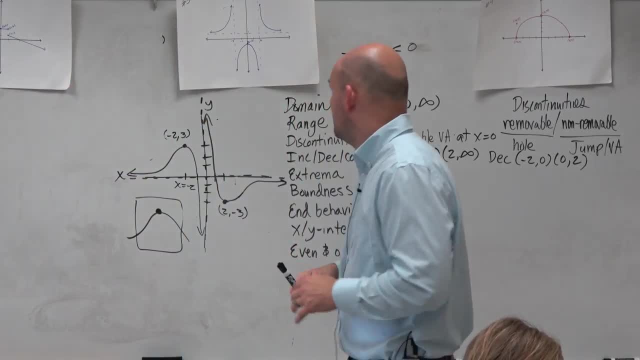 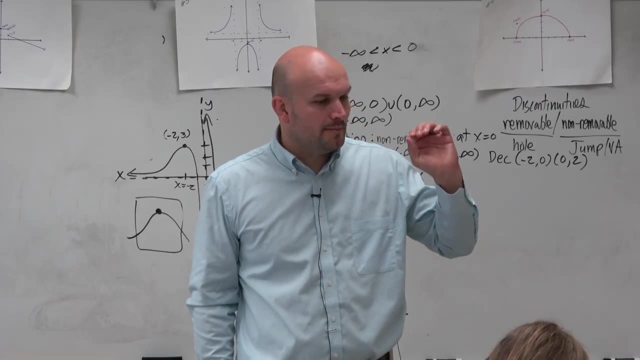 But couldn't we also say there is a maximum value of like y equals 3? Right? So the only reason I'm bringing that up is, guys, how things are asked matters, And just be careful with that, For instance, like on multiple choice Reynolds. 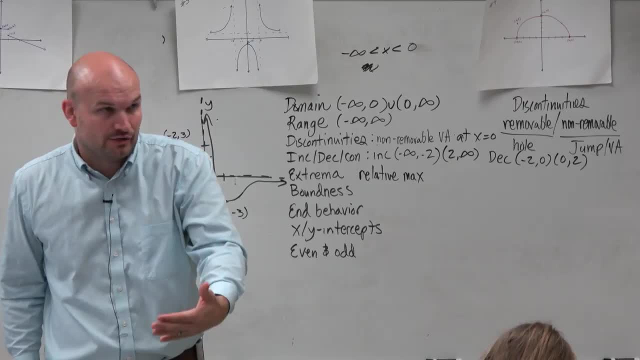 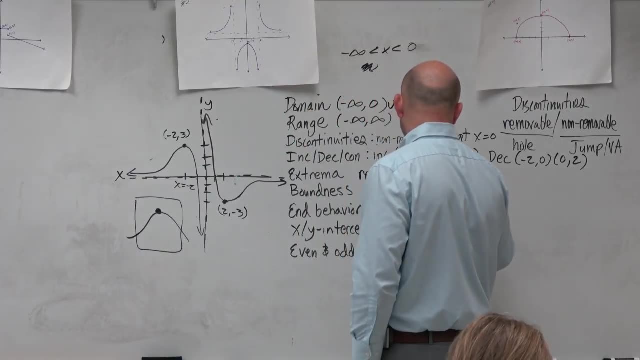 you might be asked: where is the extrema Or what is the value of the extrema. So just make sure you know the difference between what x's tells you and what y's tells you. We can also just say there's a relative max at the coordinate. 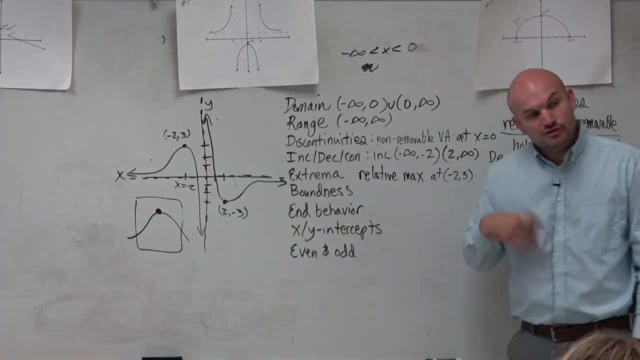 point negative 2, 3.. And using that same understanding, if I was just going to zoom in here, we would say that's a relative min And I'll just say, at the coordinate point 2, comma, negative 3.. 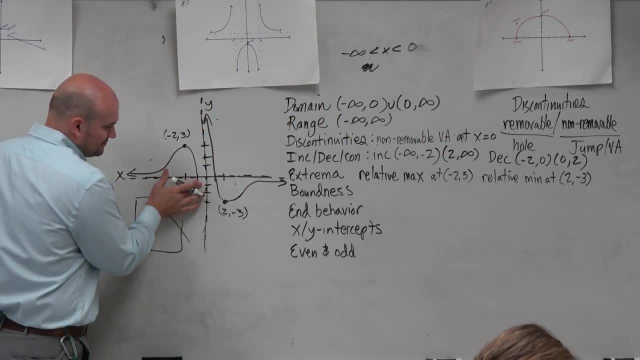 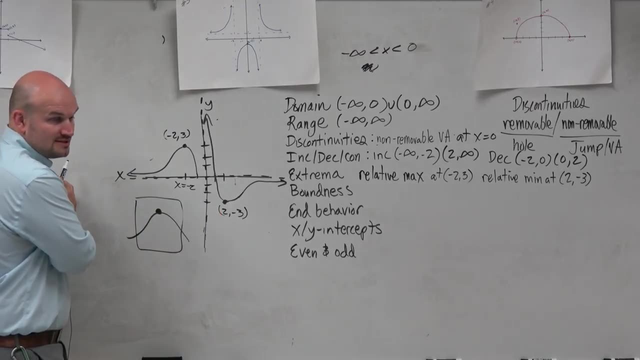 Now what if this graph stopped? Let's just say the graph stopped right now. Is this now the lowest point? Is this the lowest point of the whole graph? Yes, So when we're talking about extrema, there's relative min and max, which are just min and maxes. 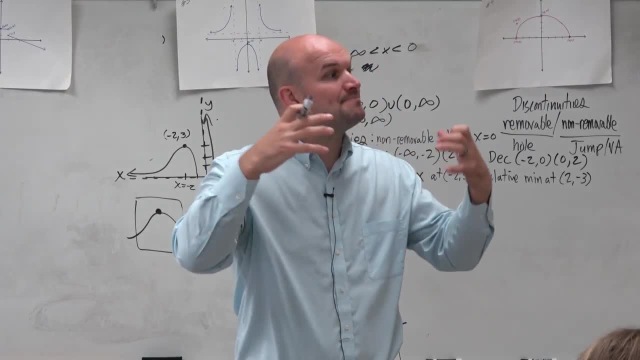 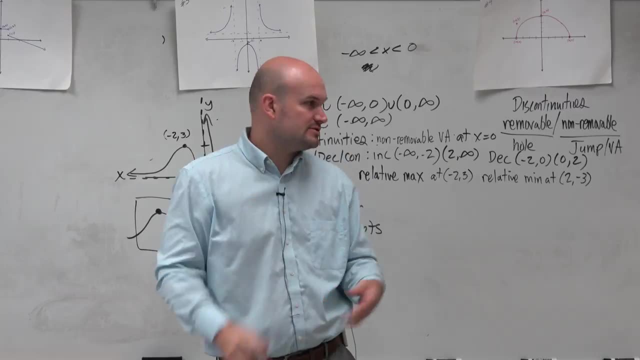 of like a zoomed in portion, And there's also absolute, And what absolute means is? it's the absolute lowest or the absolute highest? So we don't have any in this case, but I wanted to at least talk to you guys about that. 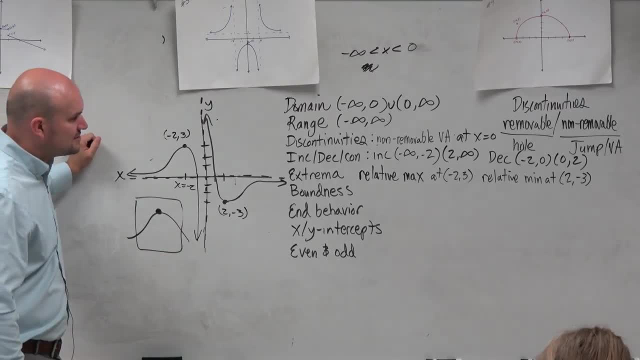 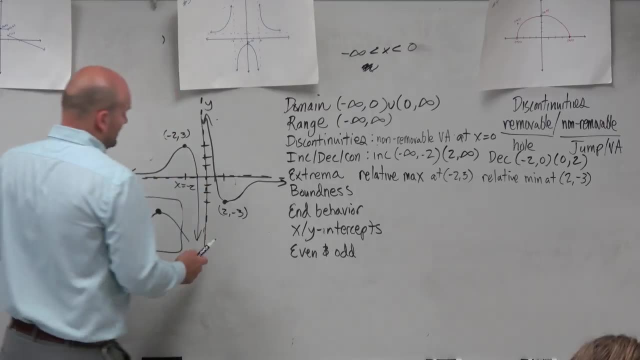 All right, now the rest of them should be rather quickly Boundness. So boundness Boundness is just really another way to say like, how is the graph restricted? So if you guys can see that this graph is continuing going up, 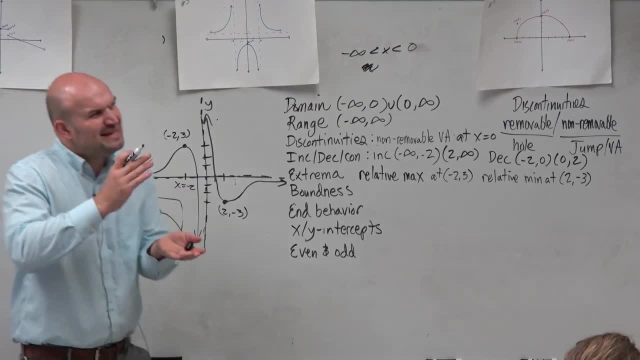 and continuing going down right. So boundness we're talking about basically like, how is the range bounded? We're not talking about the domain, We're really kind of talking about the range. Is there any restrictions in the range? 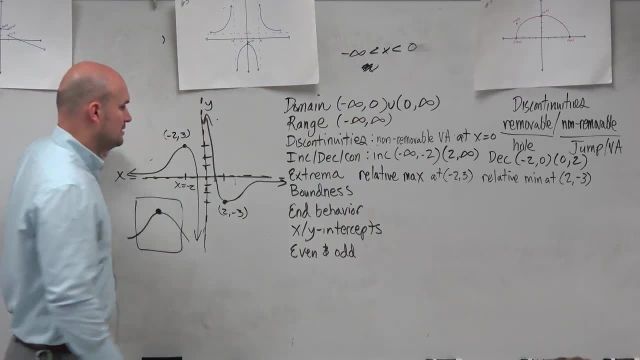 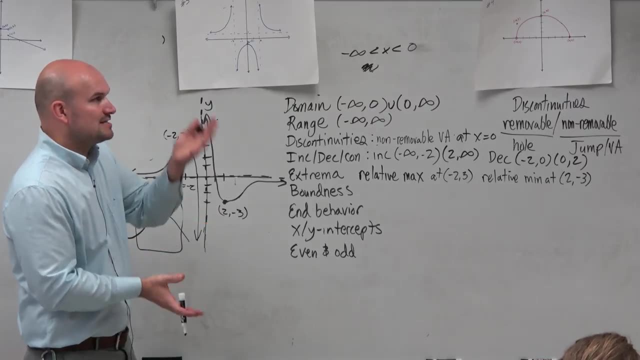 And is there any restrictions on how low or how high we're going? No, And not so much restrictions as, like gaps. I guess you'd say We're looking at the kind of like yeah, the maximum or minimum values. 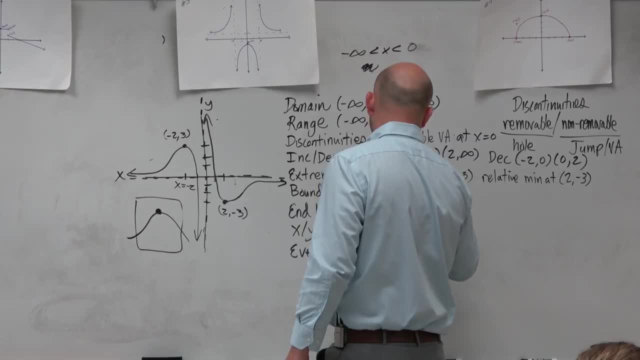 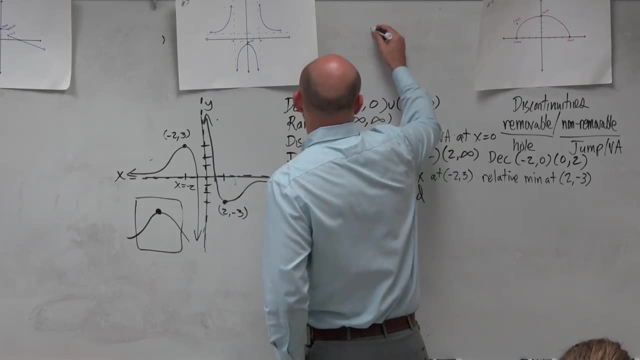 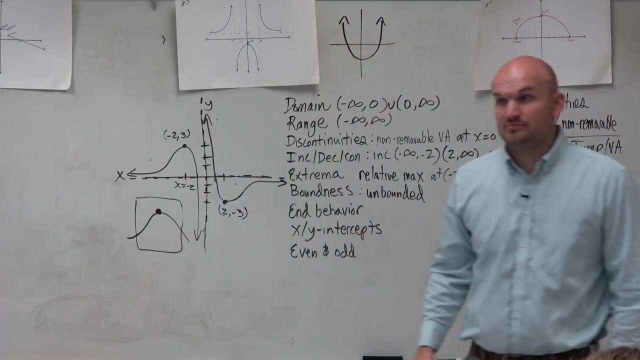 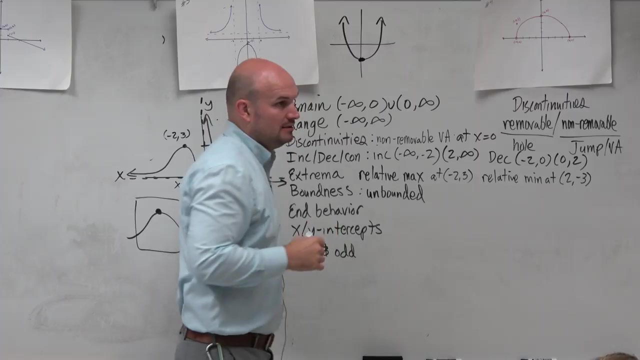 So this graph is unbounded And you might say: well then, what is an example of a bounded function? That is an example of a bounded function Because you guys see the quadratic. The quadratic has a absolute minimum value, right, What we call the vertex here. 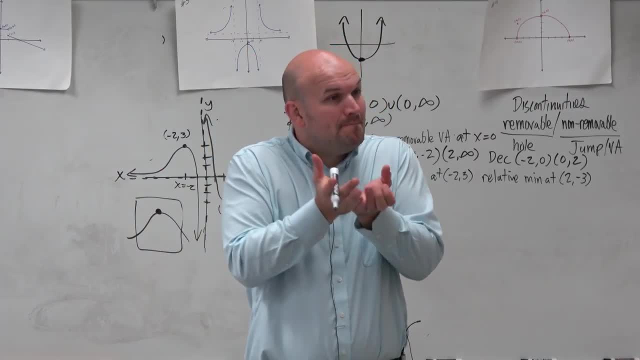 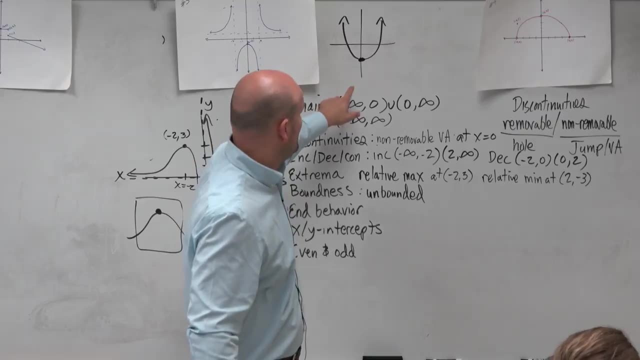 Yes, you guys remember that Algebra 2?? So that is what we call bounded, And it's restricted. You can't go below that lowest absolute minimum point, right? So this is what we call bounded below. And if I flipped it so it looked like this: 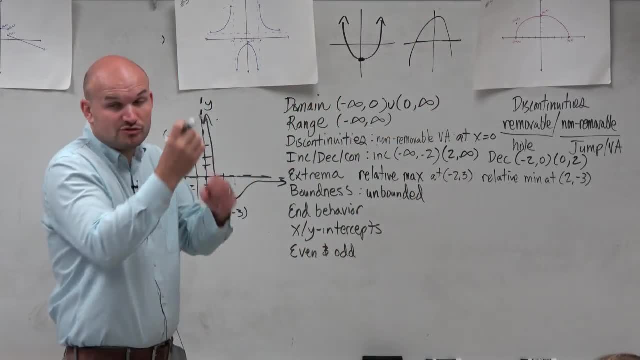 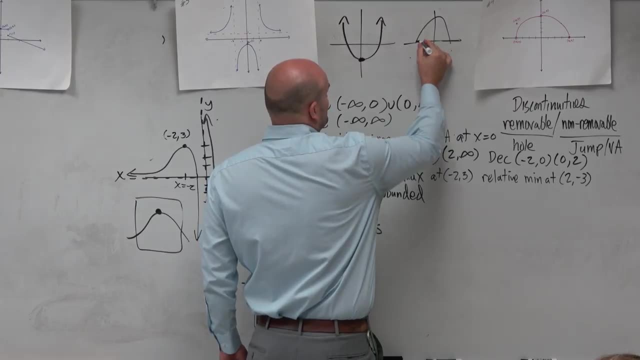 that would be called bounded above Because it's restricted, above that vertex. That make sense, And if it didn't continue like it looked something like this, we would just say it's bounded above and below, or just bounded because it's restricted. 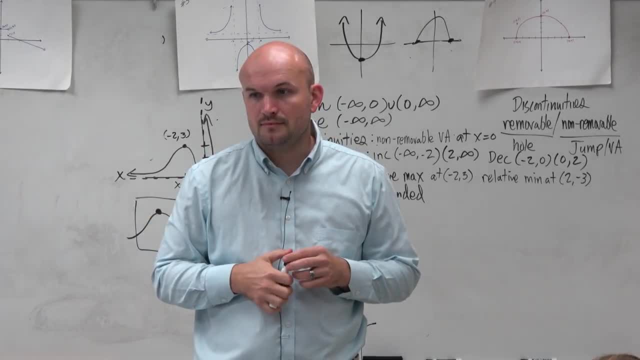 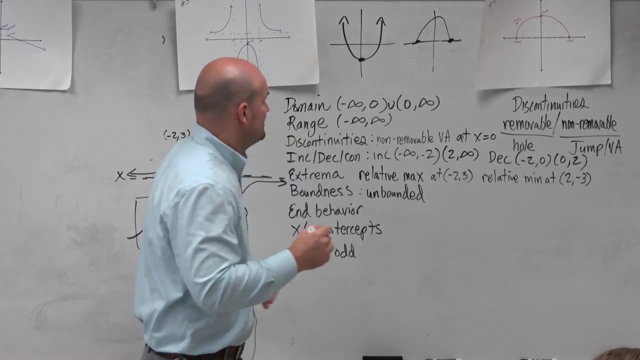 on the top and the bottom. Yes, If it's horizontal. If it's horizontal, Well, it wouldn't be a function, So we probably wouldn't be characterizing it. But again, it depends on the function. Like, if you're looking at it like this: 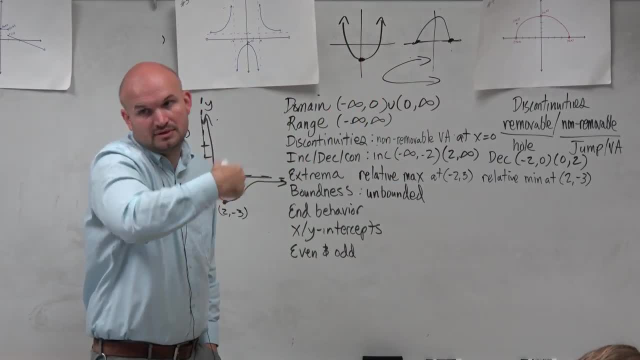 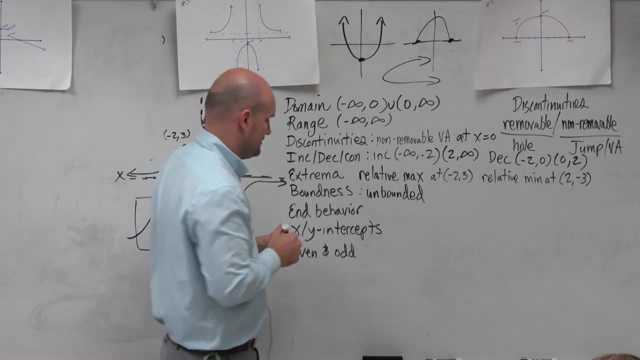 is this graph continue going up and continue going down? Yes, so technically it's unbounded, right, As long as there's no restriction on how high or how low it can go. it'd be unbounded, But for our sake of this chapter. 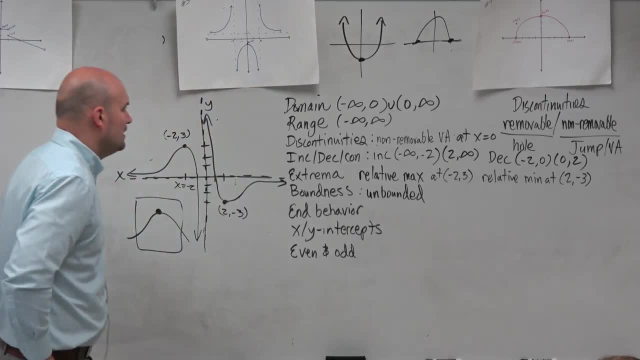 we're only going to talk about functions. so they'd all pass the vertical line test. But in this example you guys can see there's no restriction, so it's unbounded. The next thing is kind of M behavior. So M behavior is basically detailing. 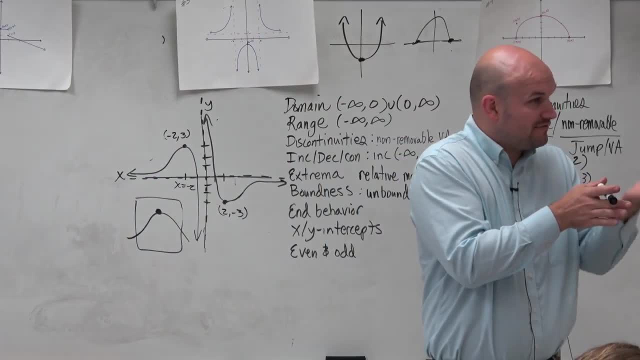 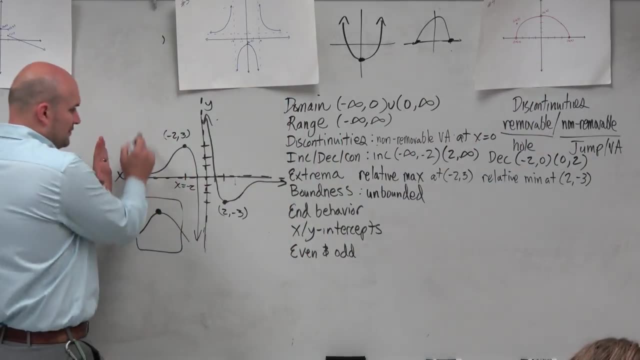 where is the graph going? So, as we move to the right, is the graph going up down or is it approaching a number? As we move to the left, as we read the graph to the left, is the graph going up down or approaching a number? 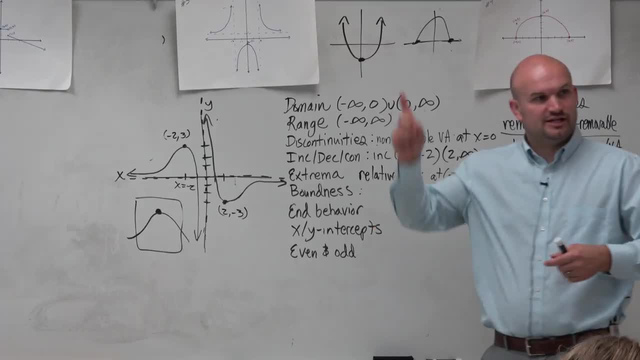 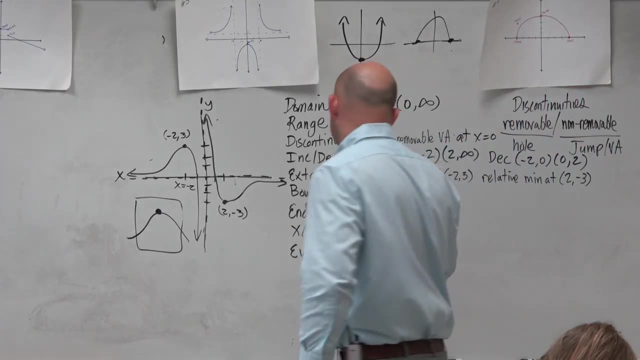 And you guys can see that the graph is not continuing up to infinity or down to negative infinity. It's actually approaching a number, right? Yes, Yes, And we'll learn a more mathematical approach here, for right now, Oops, I'm on. 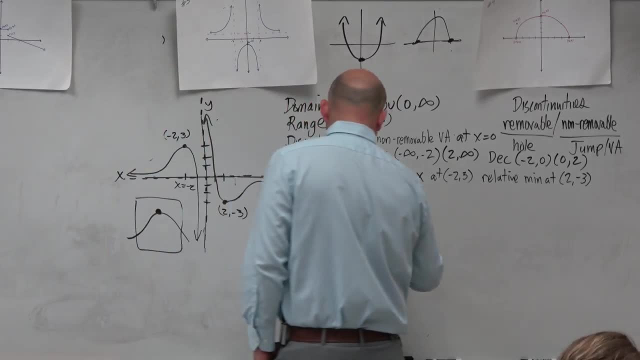 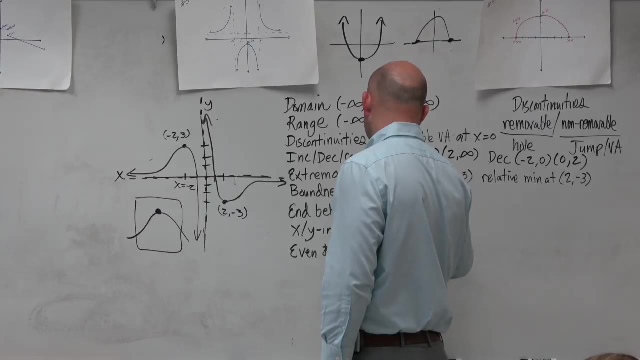 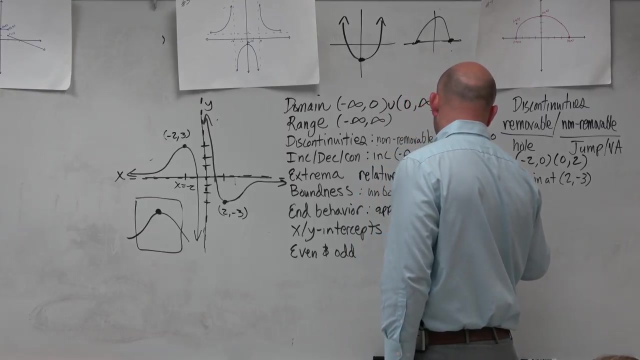 In this case we'll just talk about M behavior is going to be. the graph approaches y equals 0 from the left and right. When we're talking about M behavior, we're looking at basically as the graph expands. where is it going? 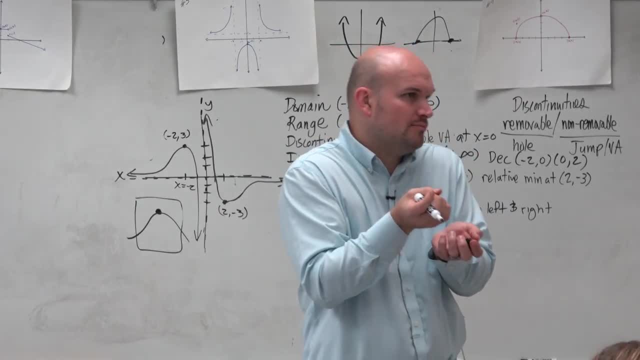 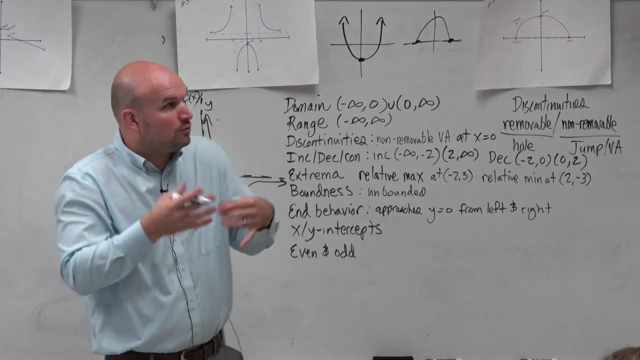 And we're looking at the y values, the output values, or more commonly often used as the f of x values, which is the same thing as the y's. But we're basically looking at M behavior. where is the graph going? Is it going up to infinity, down to negative infinity? 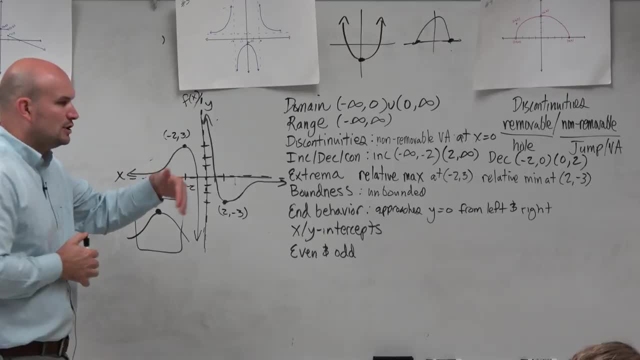 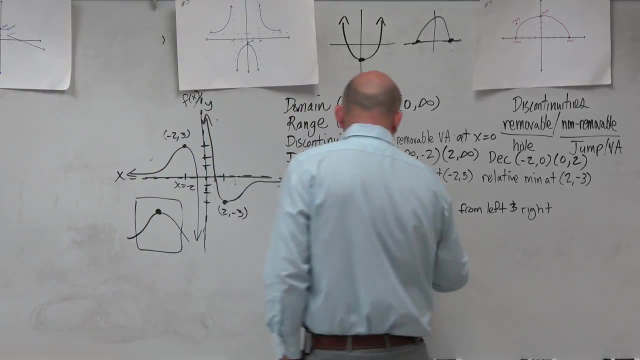 or is it approaching a number? So that's why I included the left and the right, x and y intercepts. you know, guys, we can just see that there are. There are two x intercepts. You can write the x intercepts as values. 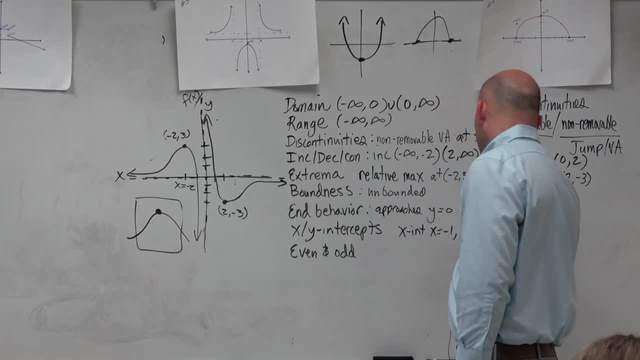 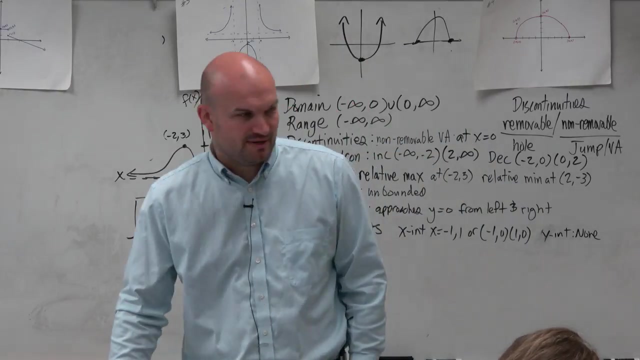 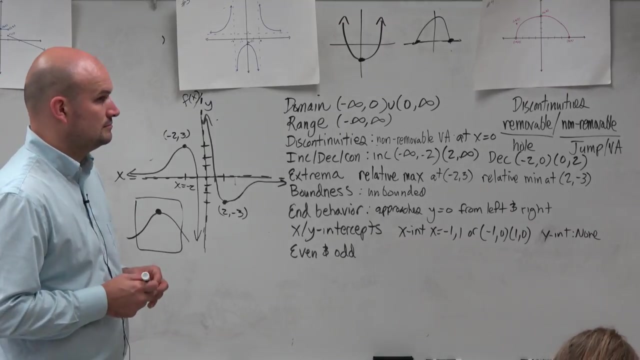 So you could say x equals negative 1 or 1.. Or we can also write them as coordinate points, And I prefer writing them as coordinate points. Yes, For the M behavior do you have to do like how you said y equals 0, how the errors are going. 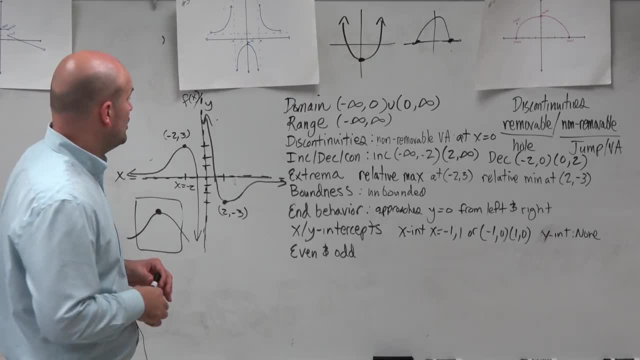 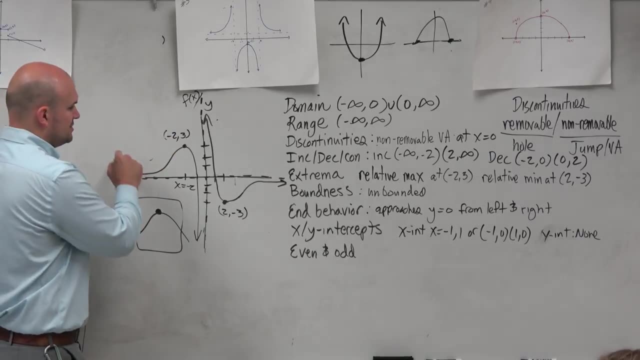 to x. Yes, Yes. So what we're saying is as we read this graph from the left and right, so just like, pretend it's like a roller coaster. So, as I continue going to the right, where am I going? Am I shooting up to infinity, shooting down to negative infinity? 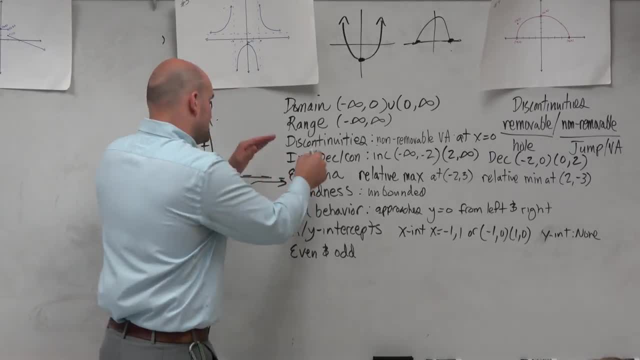 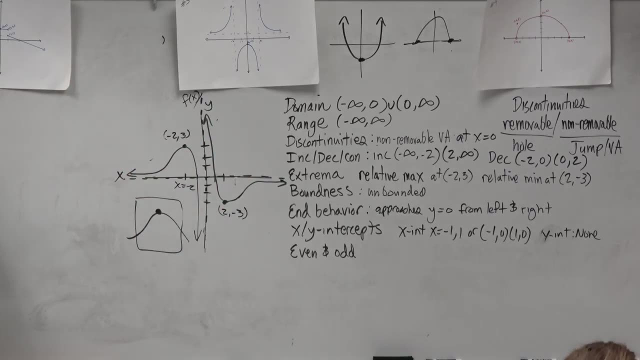 or am I approaching a number? You're approaching 0.. So as I read to the left, hop over again. I'm approaching 0.. So when we're talking about M behavior, we're looking at the expansion going left and right. 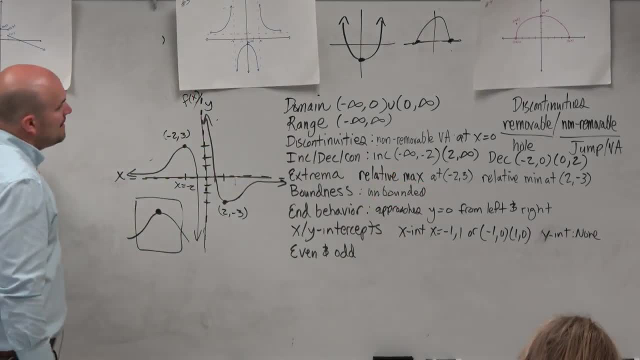 Where are you going? And basically, another way of thinking about that is like: again, here's your frame of reference. If you zoom out even further, where is this graph going to be as you continue looking to the right, or as you continue looking to the left? 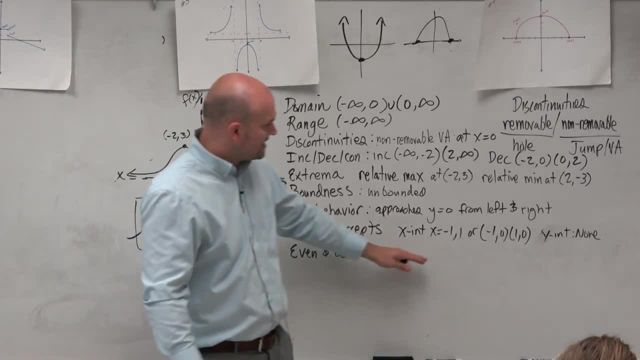 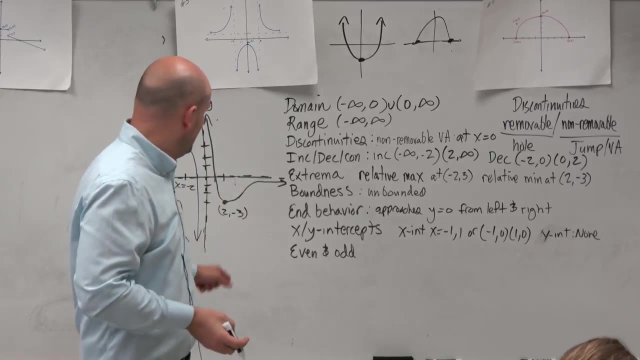 So that's kind of what M behavior is representing. I like writing x and y intercepts, though just because it reinforces the idea that y is equal to 0 when the x intercepts. If there was a y intercept, x would equal 0.. 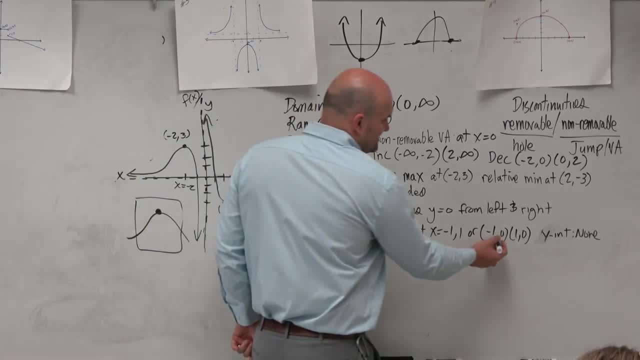 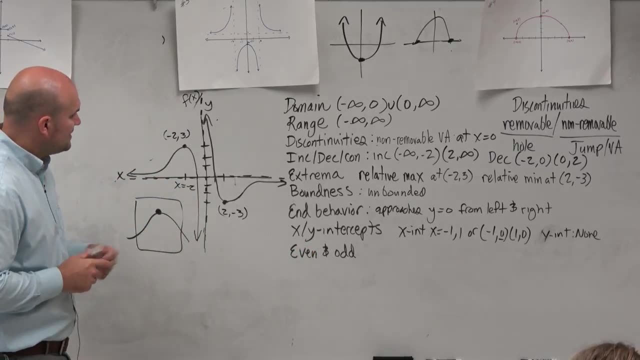 So I just like writing the coordinate points, because it reinforces this idea, which is extremely important. next chapter, that the x intercept is when y is equal to 0. And then, last but not least, is even and odd, And even and odd is basically looking: 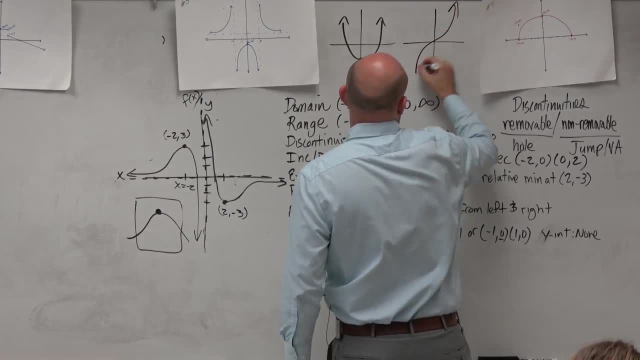 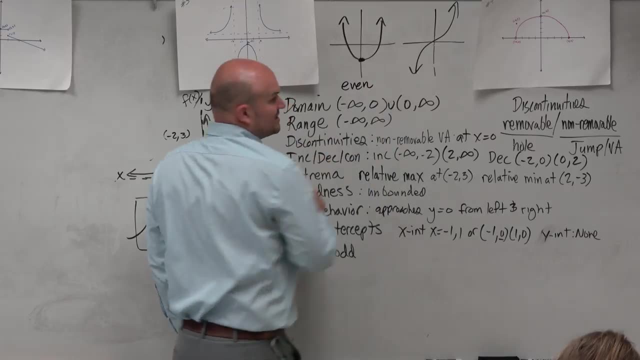 at symmetry for this chapter. So the easy way to look at this, guys, is this function is even. The reason why it's even is because it's symmetrical about the y-axis. So if you have a function that is symmetrical about the y-axis, 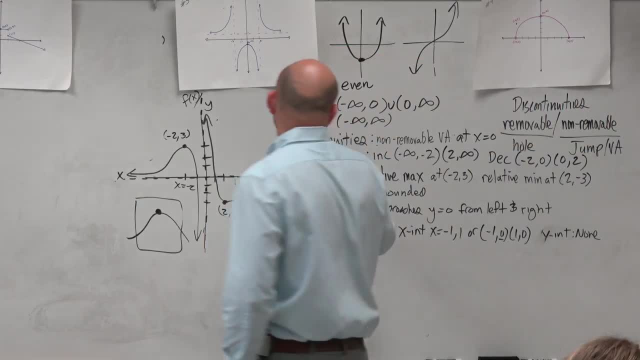 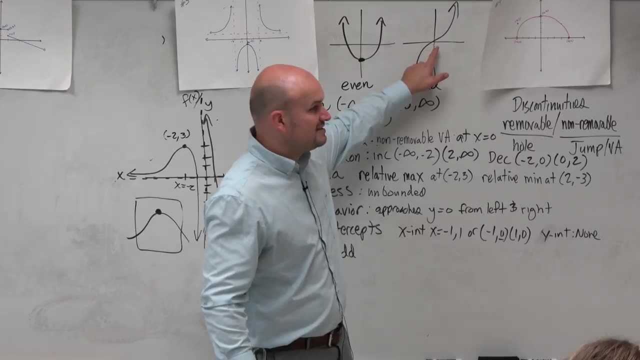 it's even. We'll talk more about why that matters later. If the function is symmetrical about the origin, it's odd Symmetrical about the origin. basically, takes this function, flips it about the y and flips it about the x. 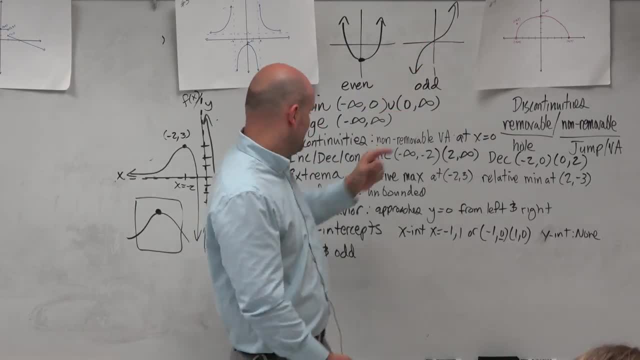 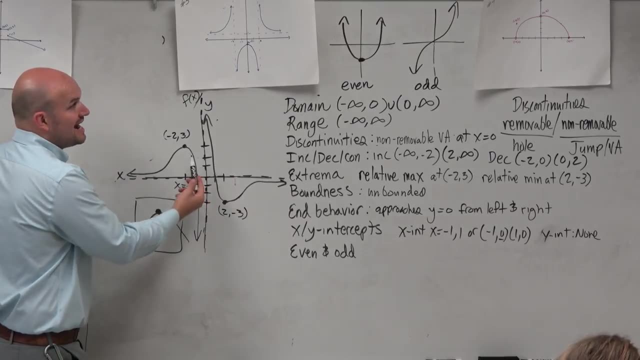 And if you can do that, flip about the y and the x. you can see it's odd. This example: is the right side the same thing, Same thing as the left side? No right? So therefore, this is not even.